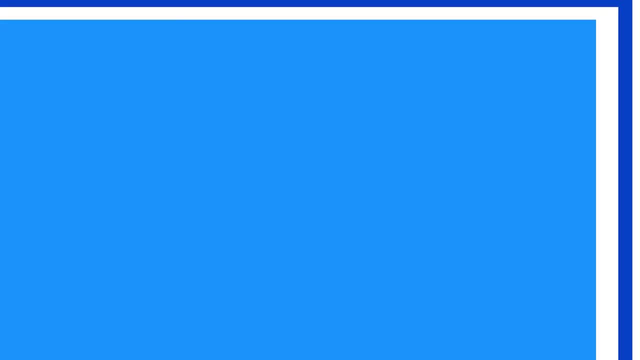 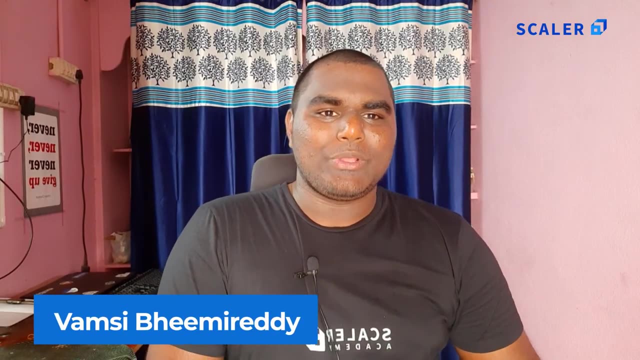 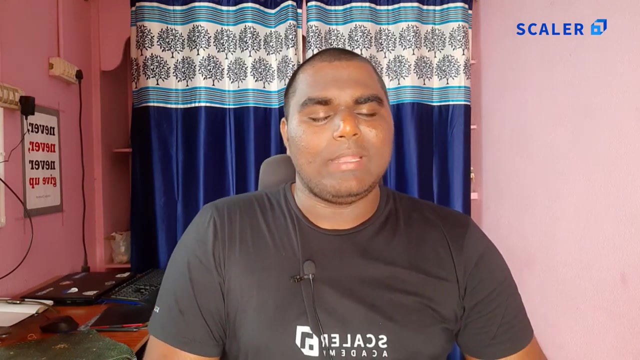 So hello everyone. welcome back to Scarlet Academy video channel. So in this tutorial we will be solving another most frequently asked interview question named longest common subsequence. First of all, we will be discussing about approach of this particular problem, and then we will be 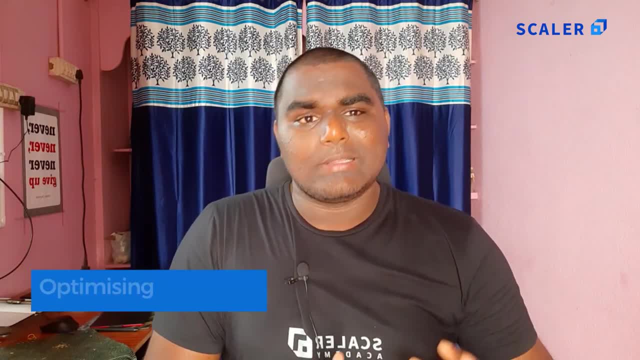 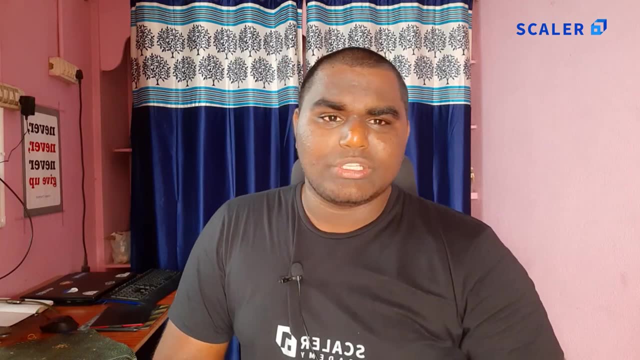 writing the recursive code, Then we will be optimizing that recursive code using dynamic programming. When I say dynamic programming, we are using two techniques, both like memoization and tabulation. So please watch this video till the end, So if you are visiting. 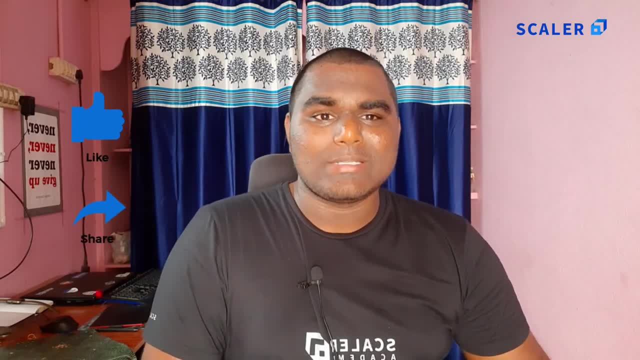 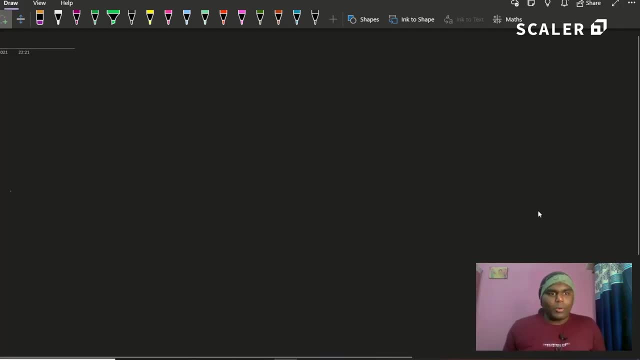 channel for the first time. please don't forget to subscribe. If you like this video, please hit that like button, and if you have any queries, please let us know in the comment section. So the problem statement will looks like this. Okay, so you will be. 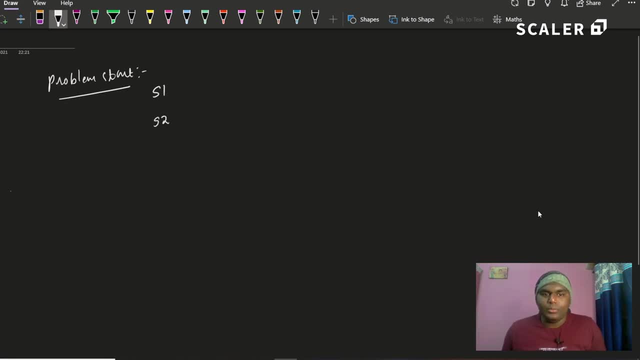 given a two strings, let's say S1 and S2.. Okay, let's say A, B, C, D, E, and another string as A, B, D, E, X. Okay, So, as you can see, the length of the strings might differ, Okay, from each other, and both are. 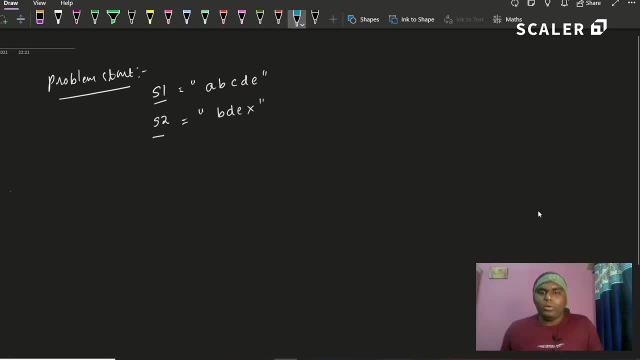 not same. Okay, And you need to figure out longest common sub sequence. When I say sub sequence, what does it mean? Okay, let's say So. in this example, let's say so: a, B and B. So here the, whatever the order, okay, let's say A and B and B. 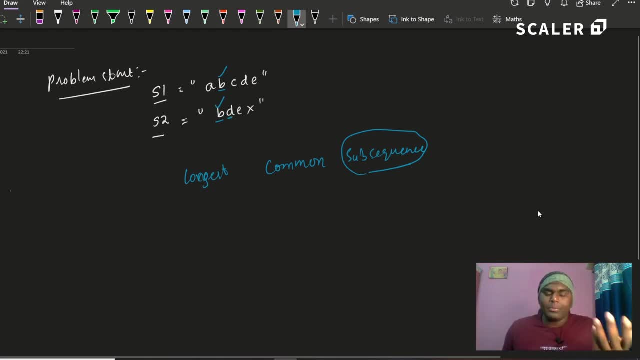 are matching. Okay, So the next element is a, D. Okay, So where does that D exist? So right after B, right, So not in order, but yes, it has occurred after B. its here, So now E, again D after So X. there is no X here, So the longest common. 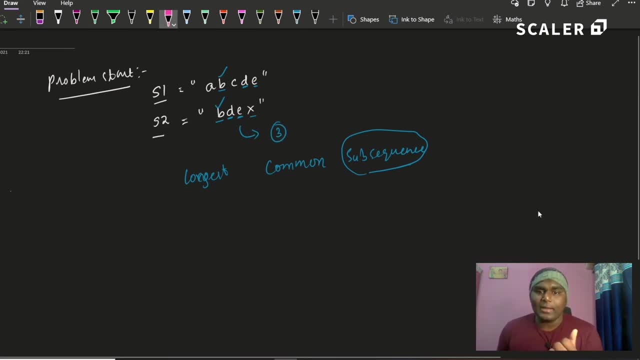 sub sequence was a 3 here. Now let's take another example, say XYZ, AB, C and here Bac. Okay, Bac. Now what is the longest common sub sequence? here B and BAC, okay, one, okay, fine, and here yeah. so both are here ba and here ab. so these both are not. 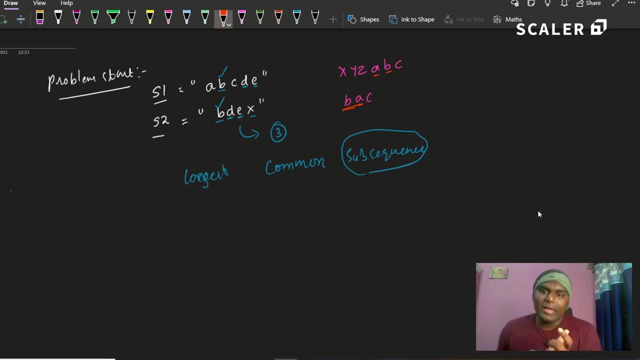 subsequence. okay, these both are not something, but individually this can be subsequence right. b alone can be a subsequence, a alone can be a subsequence right now. let's take c. okay, c here, c, so c is alone, is a subsequence. yep, so by combining the bac we do have any subsequence. 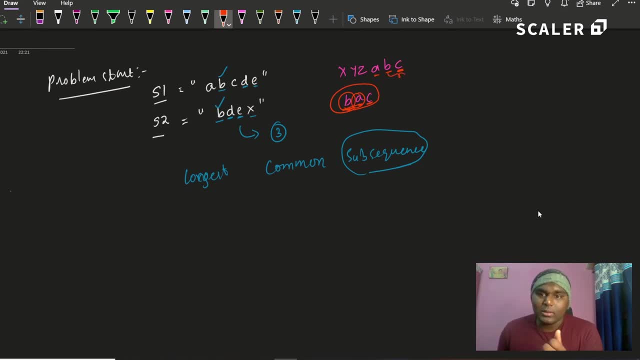 unknown. we do have any subsequence with bc: yes, two. and we do have any subsequence with ac: yes, check two. so the longest subsequence that for this particular example was two. okay, hope you figure out. okay, let me tell you another example as well. let's say a, b, c. another one was empty. 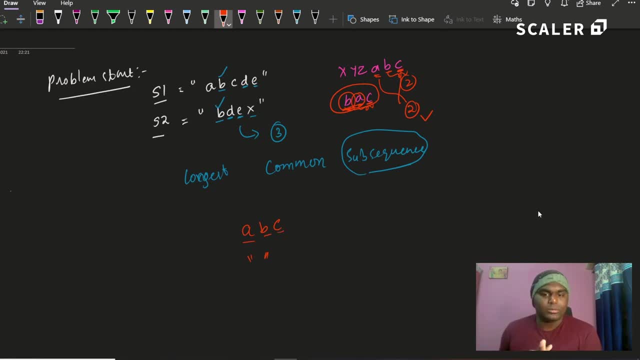 okay, okay, not, anyway. what is the longest subsequence here? so, obviously, zero. okay, hope you have understood the problem statement. okay, now pause the video for a while. come up with an brute force, approach what you can think of. okay, i will tell you. i will give you an. 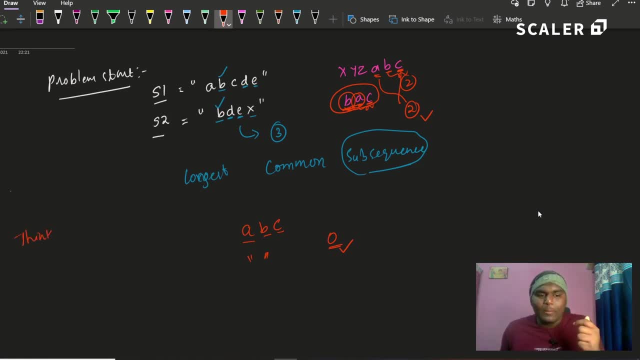 hint: okay, think in an recursive manner, recursive manner, recursive manner, recursive. okay, let's start. so we'll uh, we'll be discussing, uh, three approaches, okay, three solutions for this. okay, so, basically two, one with a recursion, another one with a dp. okay, so when i say dp, 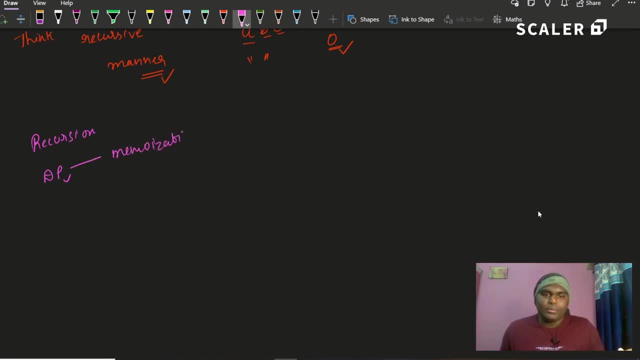 it is a both a memorization and a tabulation. what does this a memorization stands for? if you don't know what is a memorization, that's okay. fine, i will tell you. i will give you a glance about it. okay, so a memorization means, uh, you will write a. 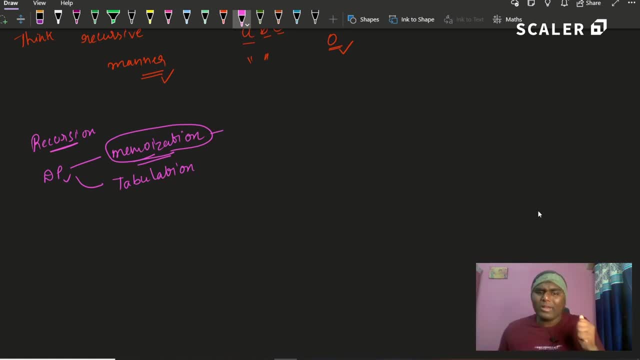 recursive code. hope you know recursion, we'll let it recursive code. okay, so you will be, uh, trying to memorize the answer which you have, um, already computed. okay, so basically, we will be having a few concepts like overlapping sub problems. okay, i will tell you what is overlapping sub problems are during our discussion, okay, of. 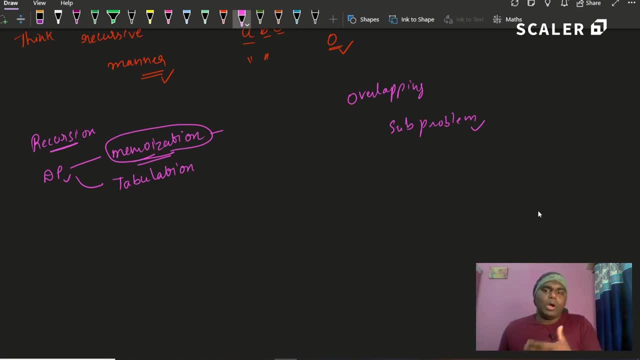 recursion tree. okay, we'll try to uh avoid that particular problem. so that is what dp stands for. okay, so using using the pre-computed value or already computed value to compute the current values. so that is what a simply dp stands for. okay, and we will be uh doing this with the recursive code only. okay, we won't write any loops here. 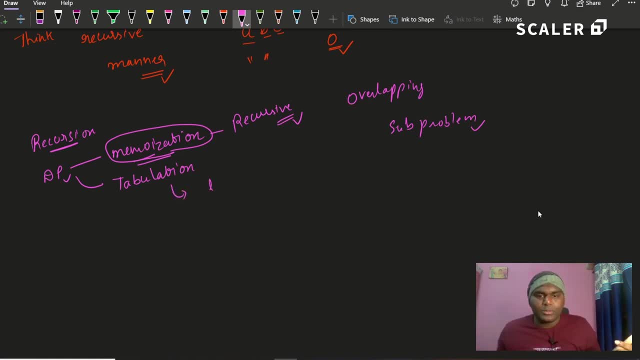 okay, but when it comes to tabulation, we will be writing a loops, okay. so basically it's an iterative, all okay. yep, this is a glance, and again, i'm using a top-down recursion, top-down recursion, so it can be done both bottom up and top down. but, um, so it's your choice, okay, what you can come up. 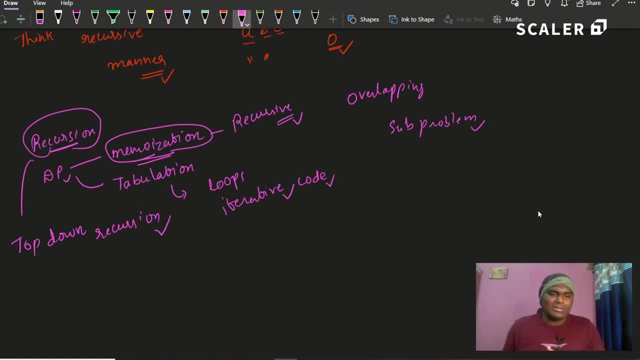 with. okay, so after watching this video you can do both things. that's not a big deal. okay, i will tell you. okay, i will write in code as well. okay, for both of these. so, without wasting any time, let's get into the solution. so first, recursion solution. okay, i will write one example here. 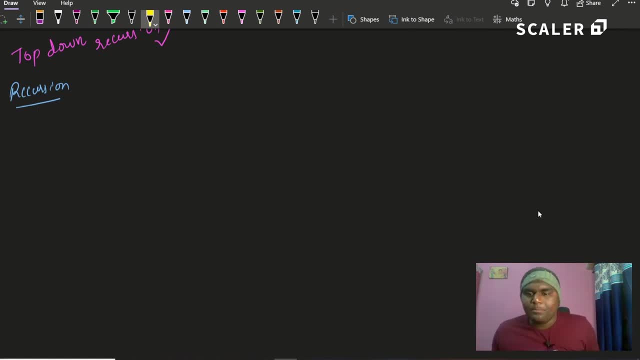 for our recursion tree. let's say, uh, let me tell you, i will pick up my name umc. okay. and let's say a s x, okay, so i will write. let me write sizes as well, indexes- okay. these are all the indexes as well. now i will try to um make an recursive tree. 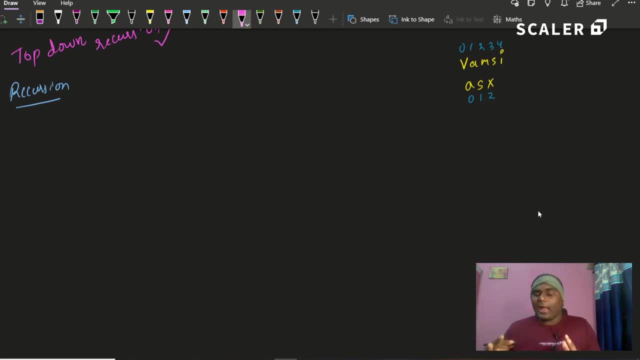 so if you don't know what is a recursive tree, okay, i i highly recommend you to watch my previous video which i have made on recursion okay, so that you will get a glance of what is the recursion tree, how to make that recursion tree, okay. so in this uh video i will be just uh going through the solution. 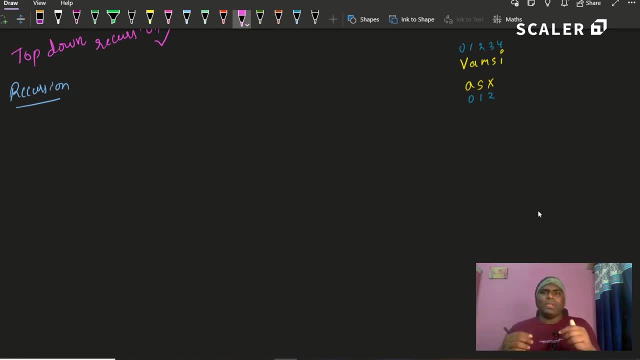 okay. so a recursive tree means, um, it's uh like a steps. okay, it contains all the steps: how i am traveling through the uh particular um like how i am traveling through entire solution. that's it, okay, in simpler case. okay, so let's say i am assuming, uh, i have an function called lcs. 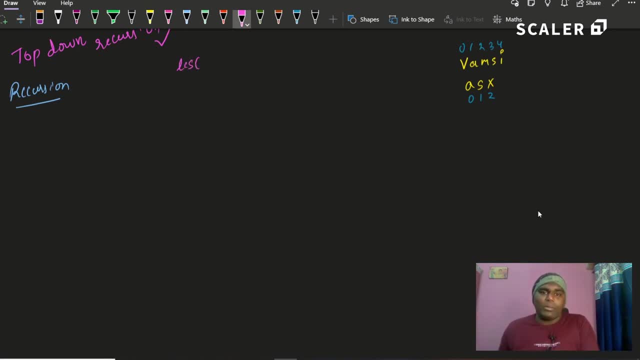 and i will be passing my indexes where i have to start from. okay, since i stated already, i am using a top down uh recursion, so i i will be starting from the bottom, okay, like start in the end. okay, so the indexes are four comma two, four comma two. now, okay, let me change my string to here: i as well. 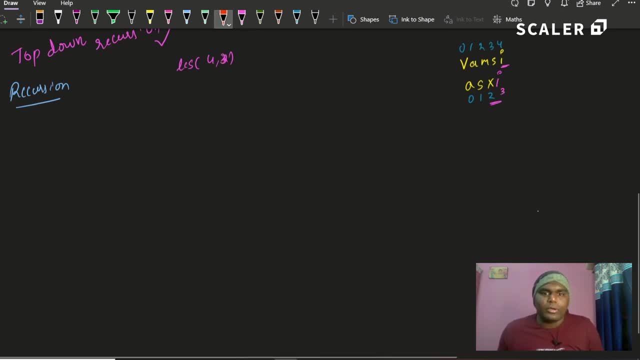 okay, so instead of three i will say four, three, four. okay, now tell me. so i and i both are equal, both are equal. so here we will be having a different cases. first case is: uh, carrot, both indexes are same. okay, so both character values, indexes are same. 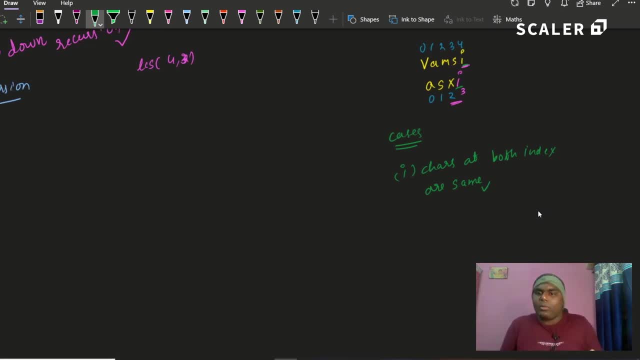 so here, okay, i will write the cases while solving the problem. okay, so, as of now, we have encountered one case, so that is both. the characters are same, so i and i. so it means that it might be my, uh, it might include in my sequence, you agree, everyone? yes, right. 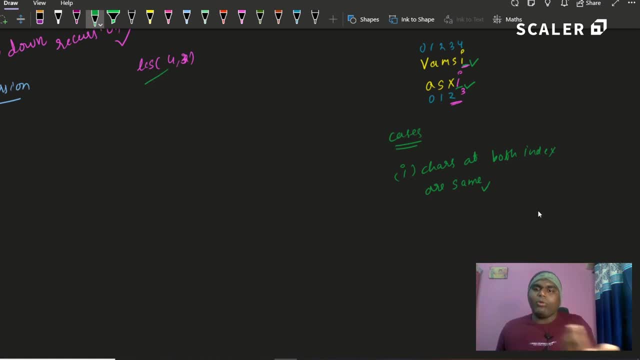 so now what i do? so i simply i have to move forward. yes, i have to simply move forward both of my pointers. okay, so i will make my index as lcs of three comma two done, done, okay, now cool. so now let's see s and x. so is both are same? no, no, so the case here was second case was not same. 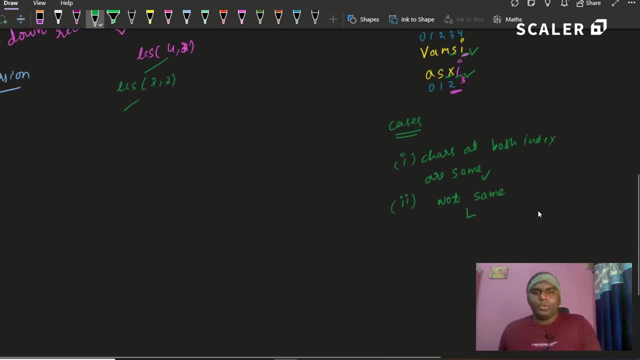 then what we need to do. so if both are not same, what we need to do? so let's say here, here, so, uh, if i increase my, if i decrease my pointer from uh two to one, two to brown, so i'm not see, i'm not decreasing my um one c's pointer, okay, it is still staying at three, only i'm just decreasing my uh. 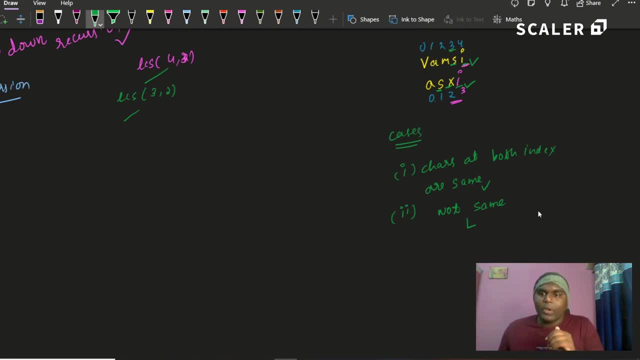 second pointer, which is, um, from two to one. now both are forming one subsequence. yes, okay, cool, so it means that i am saying that. so i have to move only one either of the one. okay, so in this case it is: i am moving second pointer, so in some cases i have to move my first. 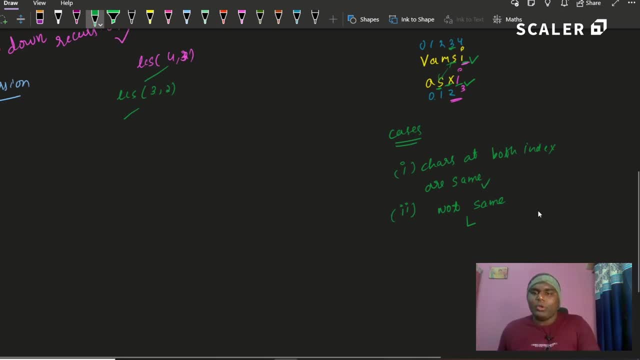 pointer as well. right, so here i will be having two conditions. so either you move first pointer, second thing, either otherwise or move second pointer. so these are the two choices i have. so basically, by when i said dp problem, it's all about choices you are going to make, okay, so now what i am doing. so 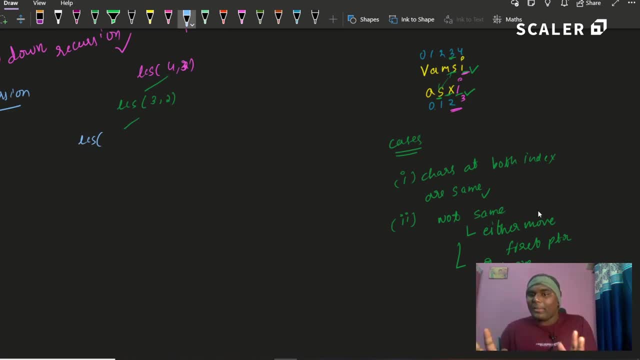 uh, first, i don't know what exactly happening over there, so i will just keep on trying all the possibilities i have, okay. so what are all the possibilities i have? no, i have two possibilities. one is move my pointer up, pointer one down, or i have to move my pointer do down. okay, so let's say, uh, first i will move my. 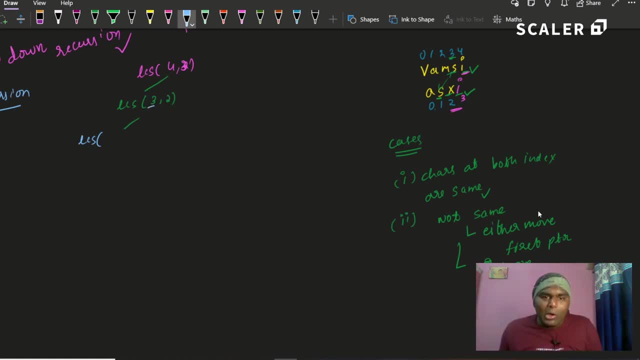 first pointer to the right. okay, so already i'm at three and two. if i move my first pointer it will be two comma two. okay, so if? if i don't want it to move my uh, first point up, i have another choice called move my second pointer, which is three comma one. earlier i am at three comma two. i have to move to three. 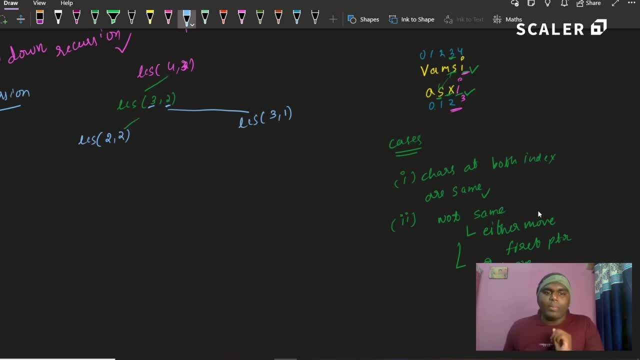 comma one. okay, done as of now. clear, okay, now let's see. so i'm at two, one, two. so m and x, so both are same and no, both are not same. again i have two options. what are all the options? so i can either either move to the right- okay, so i move my point of one to the right. let's say, if i move that one, 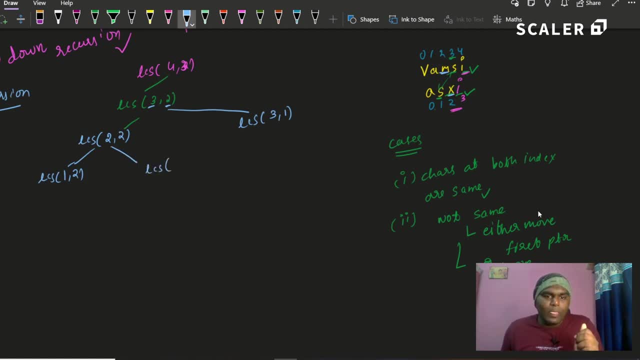 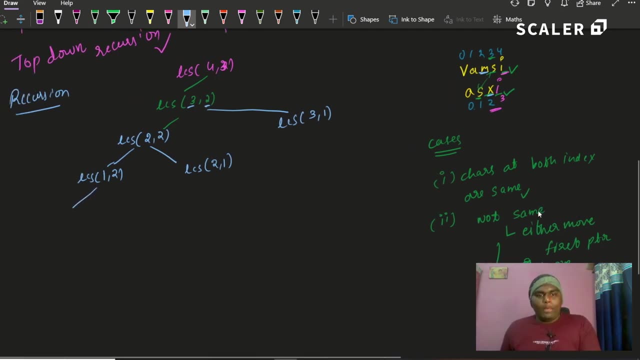 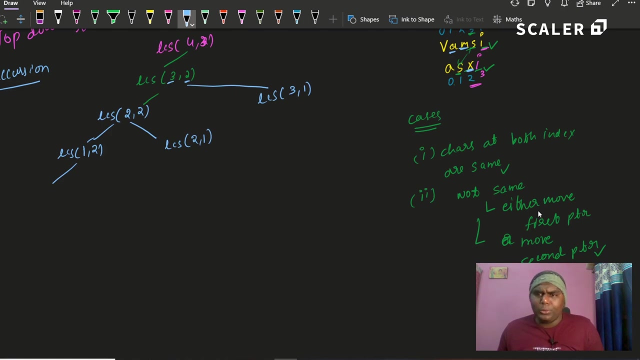 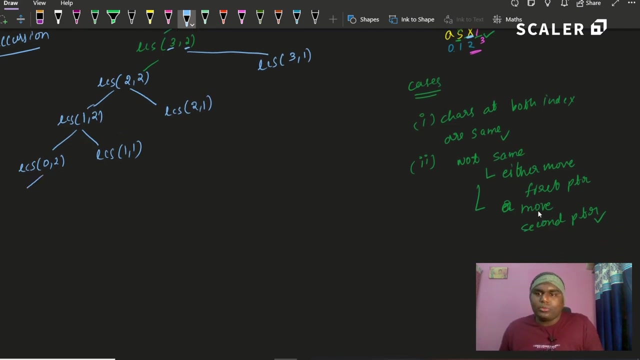 comma two, otherwise lcs of two comma one. now again, so now again. so one and two. one and two. so a and x, both are same. no, again i have two options: lcs of zero, comma two, lcs of one comma one. done so next, so again, so zero and two. uh yes, zero and a and x. both are not same. 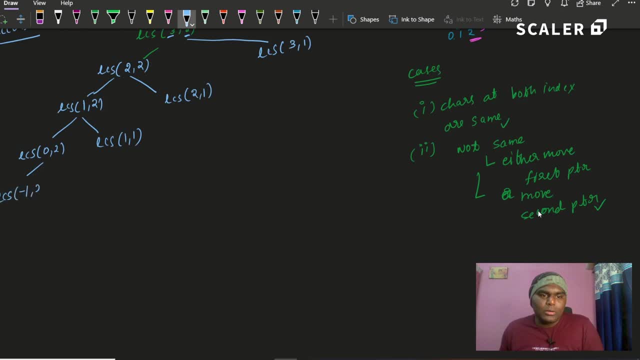 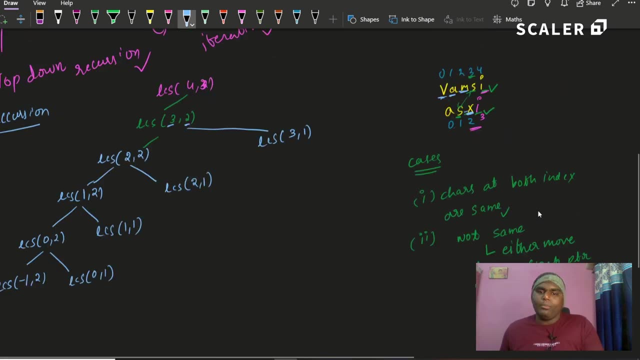 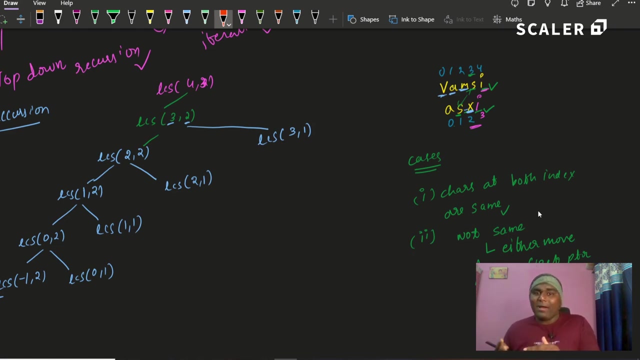 so again i have two options: minus one, two or, uh, zero one. done, okay, now i have came here. now tell me, now tell me, is there any index called a minus one? no, no, we all know that index has last one, zero only. so whenever i have came to, 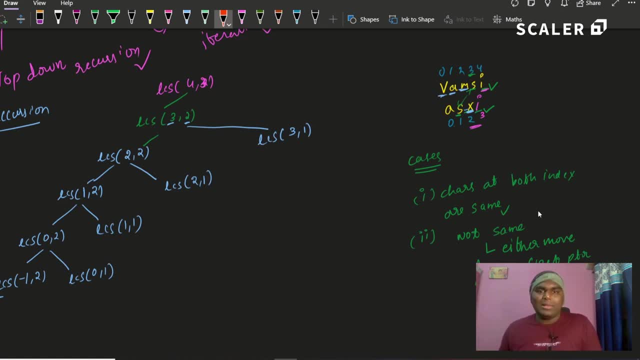 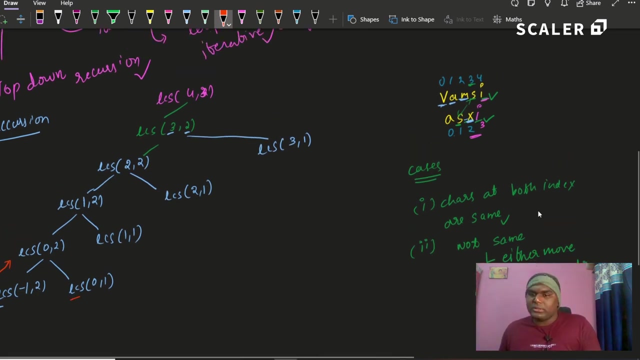 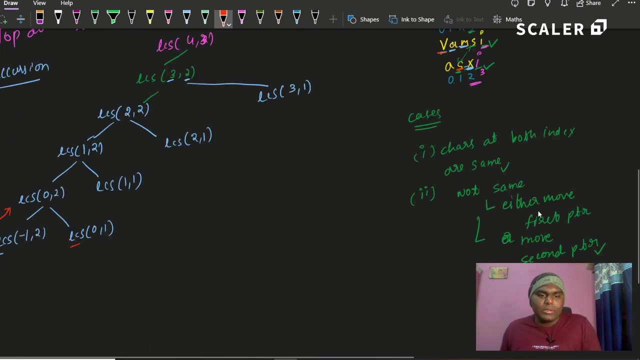 uh, index less than zero. there is nothing. okay, simply, i i will say: um return zero. okay, return zero. cool, return zero. now i have only this sub string. i will go and traverse through this. okay, so zero on one. so both are not equal. v and s are not equal. again, i have two options, less of minus one, one less of zero. 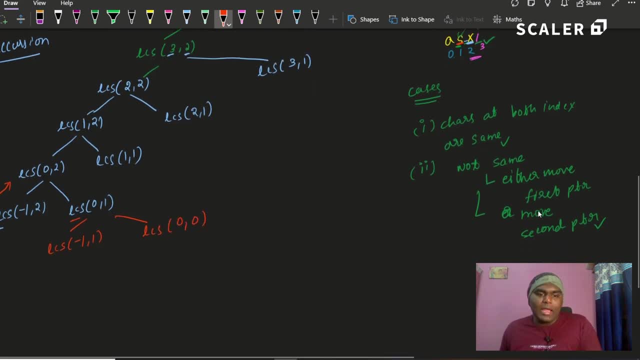 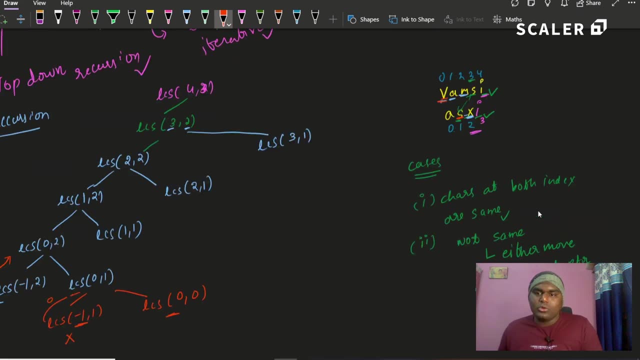 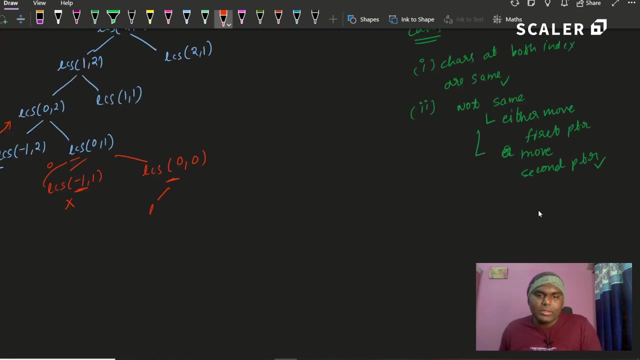 zero. okay, so again i came up with minus one. so there is nothing here. so i will simply return zero and here zero and zero. so and v and a, so both are not equal. again i have two options: lcs of minus one zero or lcs of zero comma. 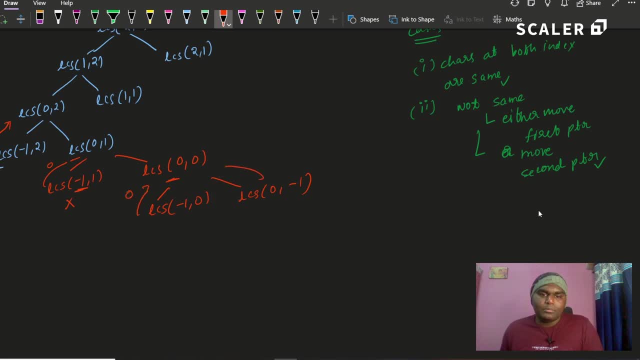 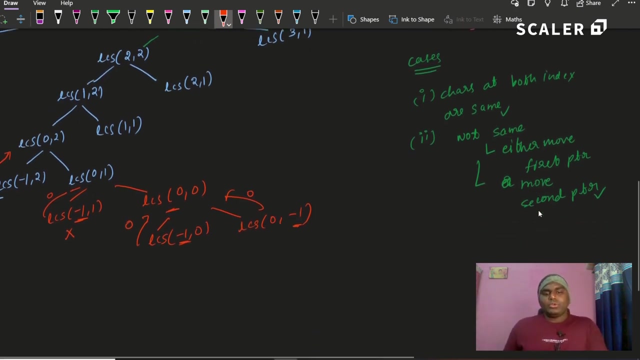 minus one. so in both the cases i will return zero, since i have reached minus one or minus one. so if either of the indexes are minus one, i have to return zero. okay, now done. done with this and done with this. now. now what next? so here i am returning some values, so i have to return zero. 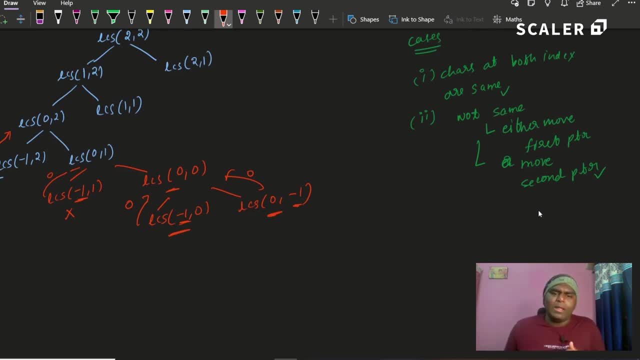 so which one do i need to consider? let's say, uh, in one of the one of the sub three. okay, either right or left. i got one sub sequence, since i am looking for the longest subsequence, what i can do, since i am traveling from the end, or if you are, it doesn't matter if you are starting from the start. 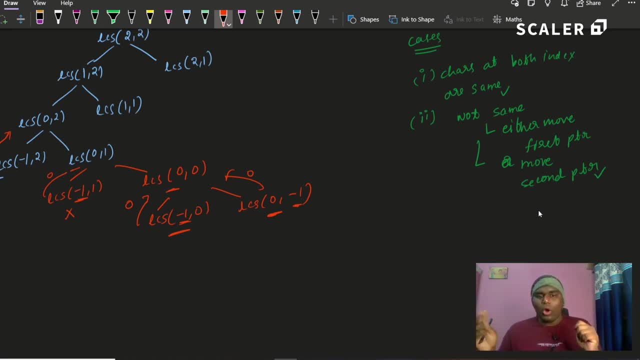 as well, doesn't matter. so if i got any subsequence, which one do i need to return? so i need to return a max of zero, uh, anything right. so i am pretty much sure that in one of the ways i will definitely reach a zero, right, if one of the ways i will definitely reach zero, because that is a base. 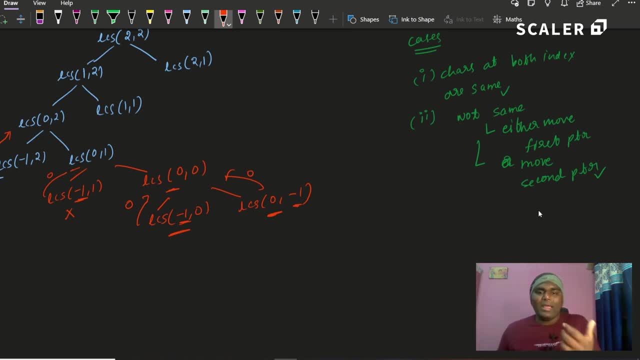 case, that is what you will end up with. okay, so if i whatever, if i get anything at the right hand side which is a greater than zero, or let's say one and two as well, so i have to consider longest, longest, so i need to consider a max. so here i will return. 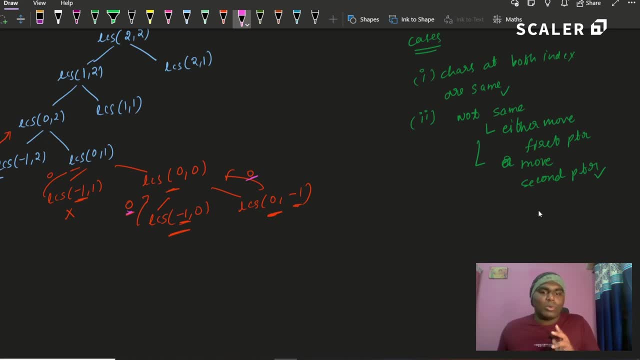 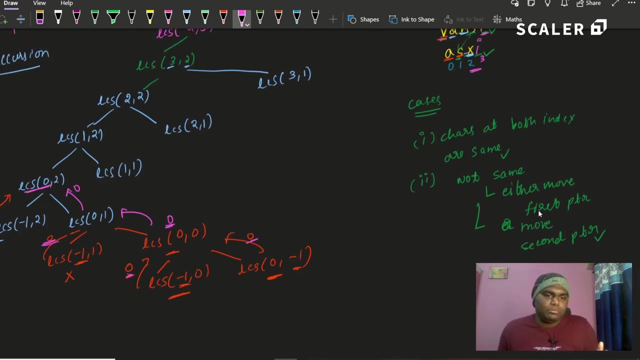 max among both the subtrees: right max among both the subtrees. what is the max among both? so zero, okay, i will return zero here. so again zero on zero. i will return max. so again it's a zero. now it has max. okay, so zero. so it will return zero. now i have to solve this particular sub sequence. 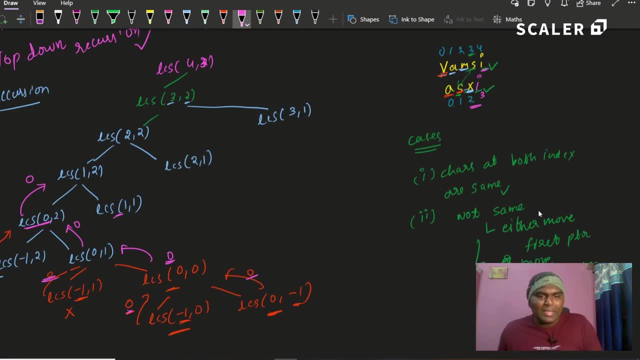 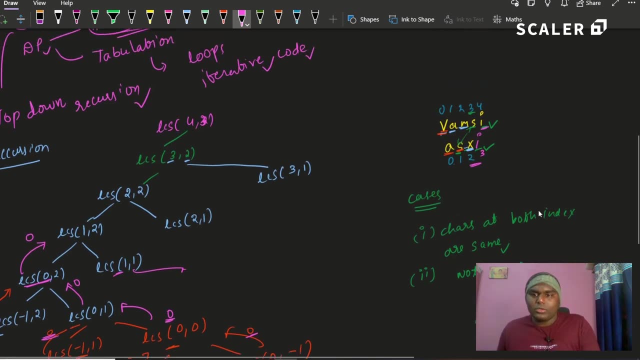 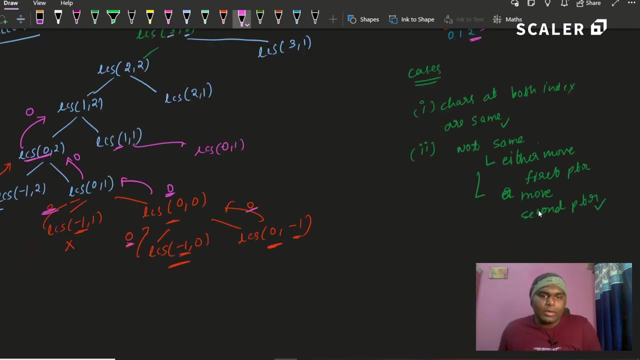 okay, uh, yeah, there is no space at all. let's see. okay, so uh, one and one, so a and yes, both are not equal. yes, lcs of uh 0, 1 and another one was lcs of 1 comma 0. okay, so we know the answer of a 0 and 1 right like here. so we are 0 and 1, both are not. 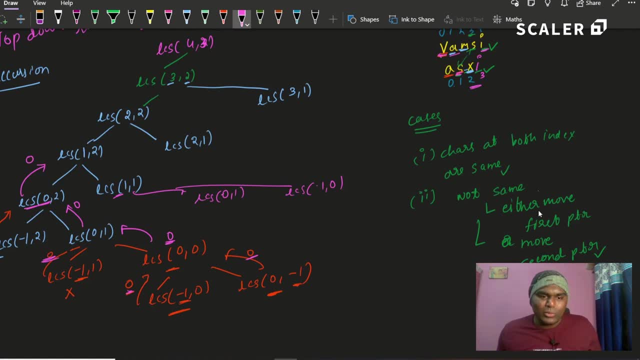 equal, so it will return 0 only. okay, since we have computer, since we have, we don't have much space, i'm just utilizing that. okay, so 0, and i will return 0 here in this case as well. 1 and 0 did we computed that? no, okay, let's see. so here 1 and here 0, so a and a, both are equal, a and a. 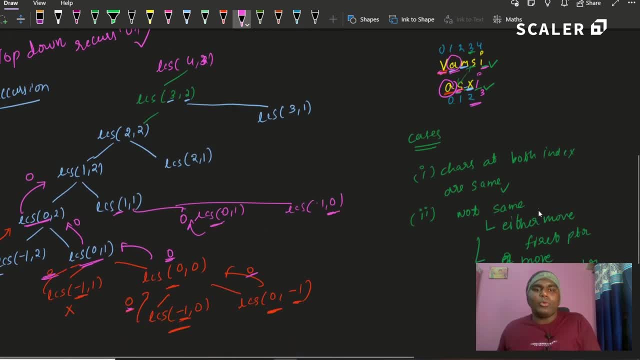 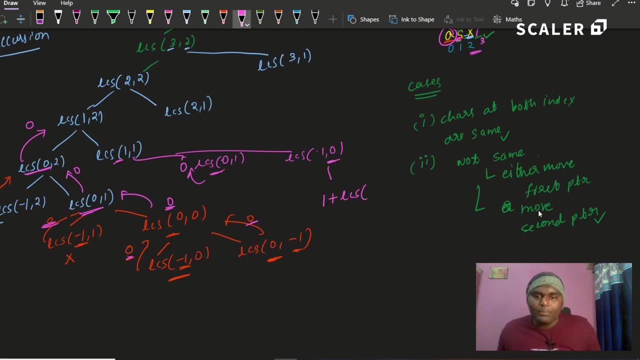 both are equal. it means that you have to compute 1. okay, you have to return 1, you got something right. so it means that we have to make another call with 1 plus lcs of you have to decrease both. you have to move a forward like you have to come to down. okay, so a 0 and minus 1. okay, so we have. 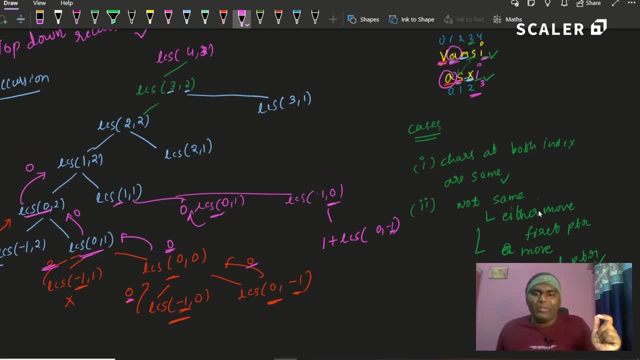 seen a minus 1 in one of the cases, so we will return 0 here for this thing for sure, okay. so 1 plus 0, it says 1. okay, we will return 1 here. and per right side 0, left side 1. so what i did what i told earlier: you have to return the max, max, max. 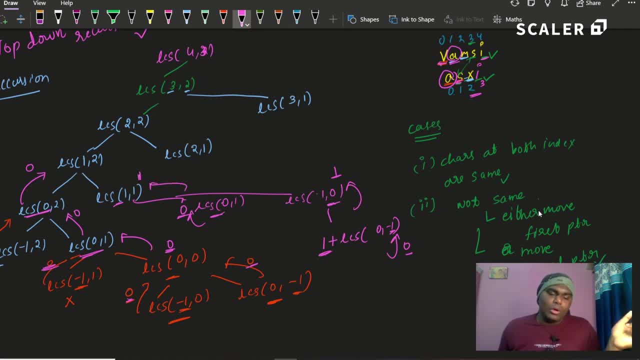 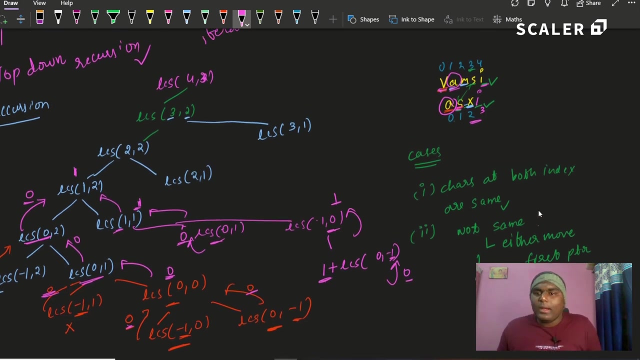 right, so you will return 1 here. so, uh, here you have 0 and here you have 1, so you will consider max 1. now let's go and solve this particular problem. so 2 1 1, what is it? 2 1 1 as a 2 m and. 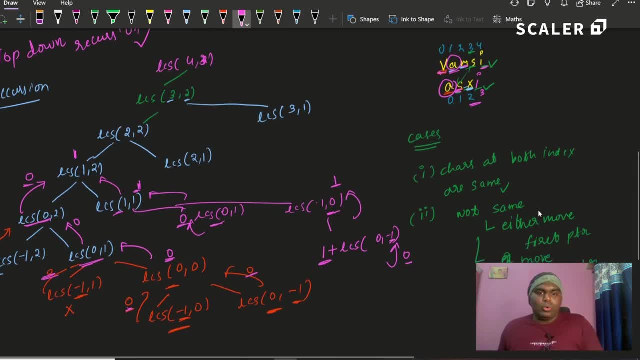 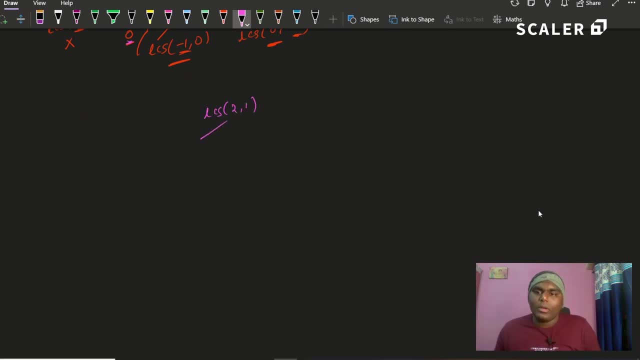 1 as s. okay, so, so, so, so, so, so let me draw that to lcs of 2, comma 1 here. okay, yeah now. so let me write the indexes: 0, 1, 2, 3, 4. 0, 1, 2, 3, okay, so 2 1, 1. 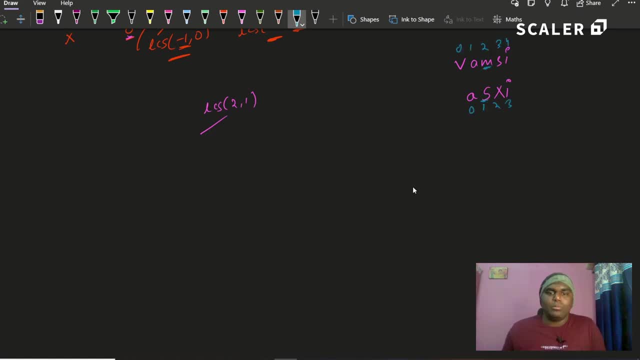 yes, 0 now if i do one and one. so 1, 1 months. sorry again, yes, but to not equal to what i can say. so, uh, again, i can move is a left you can move? okay, again, okay, but you can also do if you go to the left side i can do a more left i can remove. 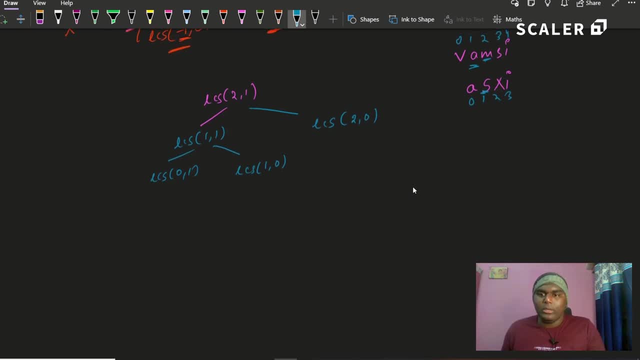 okay, so 0 and 1 again. both are not equal, so lcs of minus 1 comma 1, lcs of 0 comma 0, so it will return 0, since you have no minus 1 index. okay, now again, 0 and 0. both are not equal, so you will. 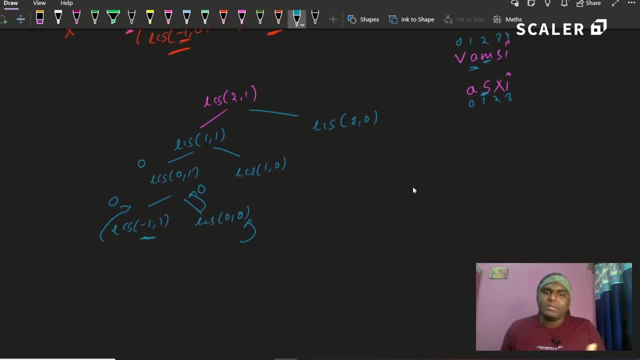 return a 0 again, so top is a 0. now you will go on this side and 1 and a 0, so both are equal. so you will return 1 and you will go to our next index, 0 comma minus 1. so we have seen minus 1. so 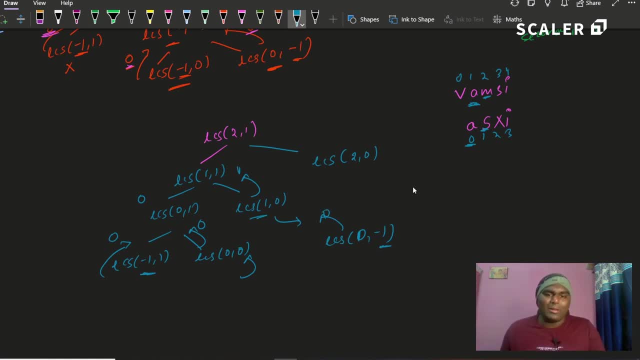 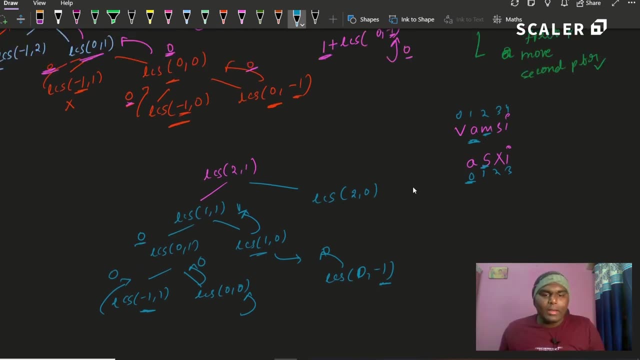 again if we return 0 only. so that's why i have directly written minus 1 here. okay, sorry. plus 1, okay, sorry. so now again, max among this was 1. now i will traverse through this lcs of 2 comma: 0, 2. 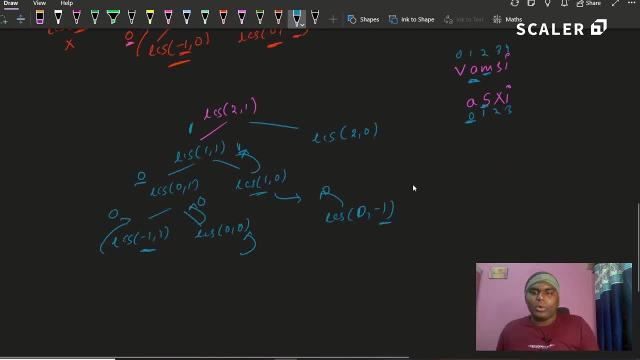 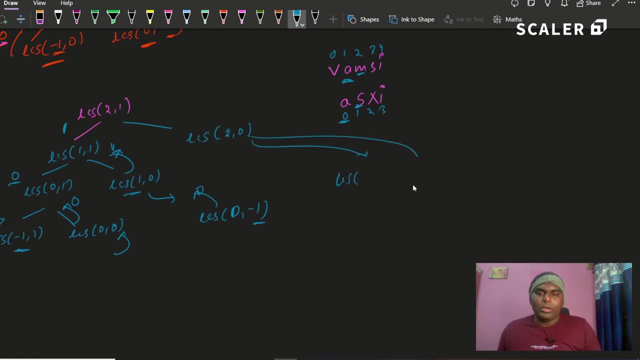 comma 0, m and a, so both are not equal. what you will do? so you will decrease these things, okay. so, lcs of 1 comma 0. lcs of a: 2 comma minus 1. okay, so, since you have seen minus 1, it will be returning 0 only and here 1 comma 0, so 1 and 0. yes, it has seen. 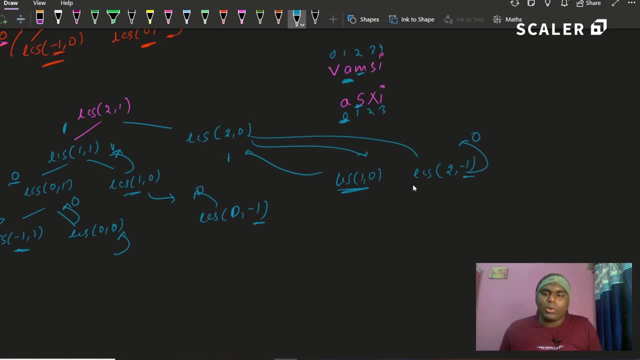 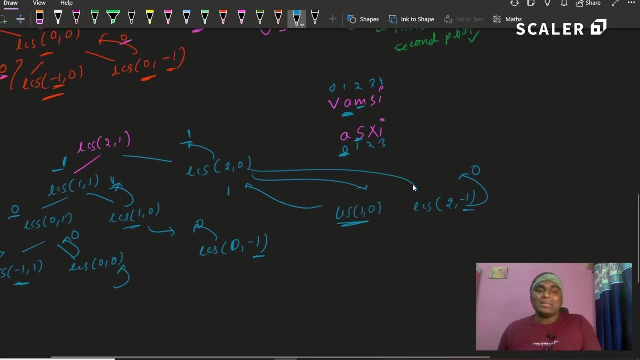 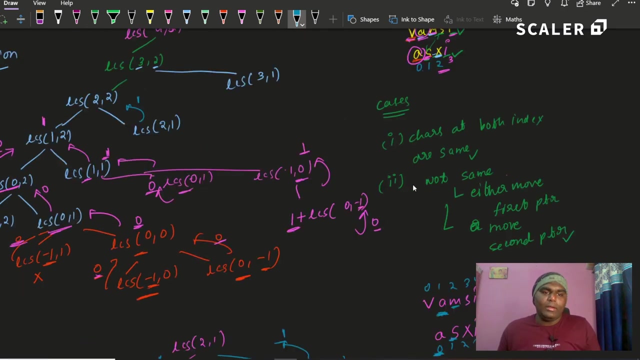 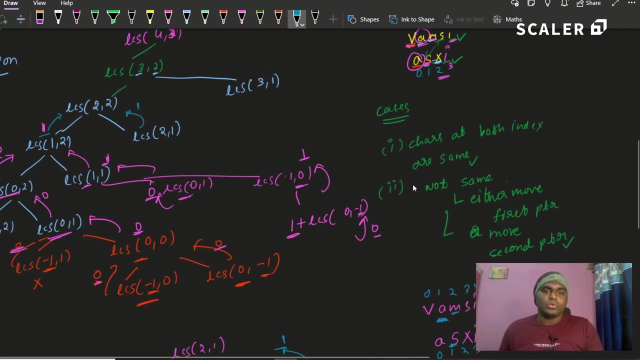 yes, 1, so it will return 1. so max among this, 1 and 0 are 1, so max among this was 1. so it means that lcs of 2 comma 1 is returning 1, returning 1. so here uh, lcs of 1 comma 2 returning 1. lcs of 2 comma 1 returning 1. so max among this: 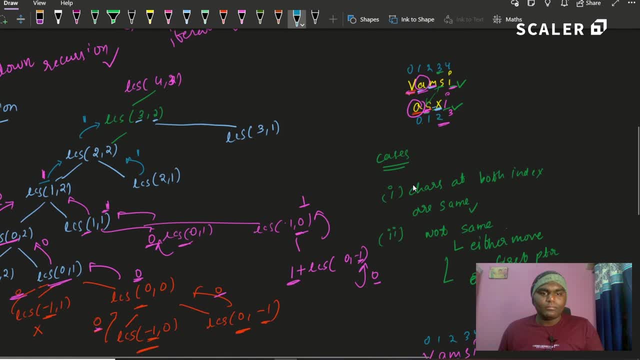 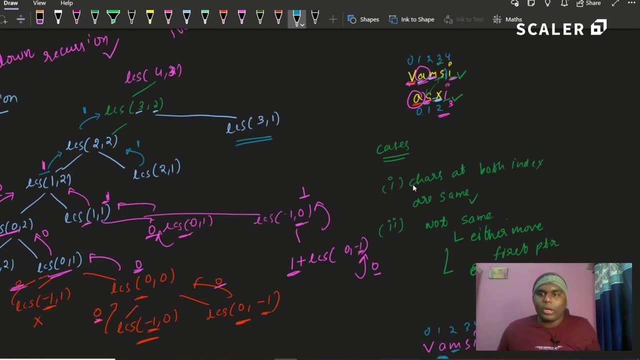 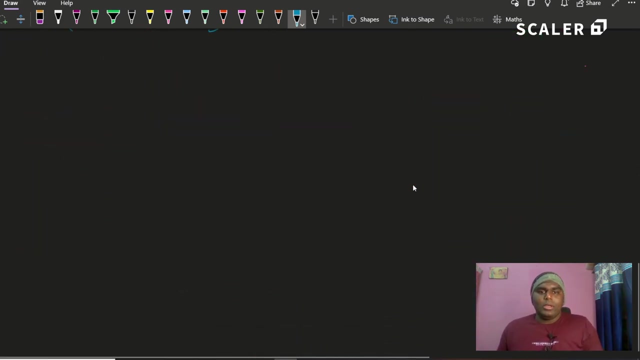 was 1, so you will return 1 here. now your job is to calculate for 3 comma 1. okay, 3 comma 1. okay, let's go and see this lcs of 3 comma 1. so 1c. okay, yeah, is that this one? okay, sorry, yes, okay now. so 3 and 1. 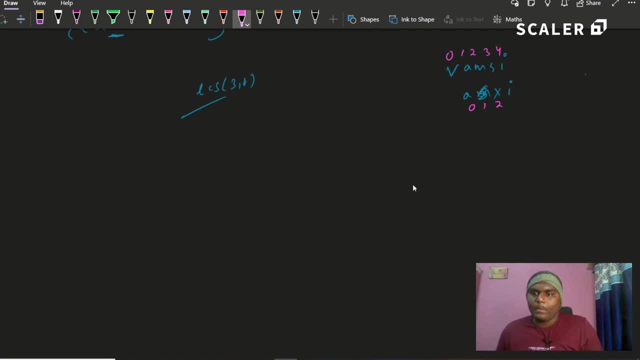 so 3 and 1 not equal to 2 and 1 device. do not do this again. so 3 and 1, right. so we have esa, three rc s in total: 1 cция of three rc s. so 3 and 1. so 3 and 1, three rc s in total: 6. in total 5 c. Daar are examples what we have said in the lesson. so kala eighth number is n plus 1 double kommeni. so these have same thing. you have to go again these 다음 and two exceeds kala eighth. we are going to correct theательно policy n here they have showed. think that if you change our patient, which will prepare the function like the other side and this results, you will not show how this will look good in the code. be went to check. 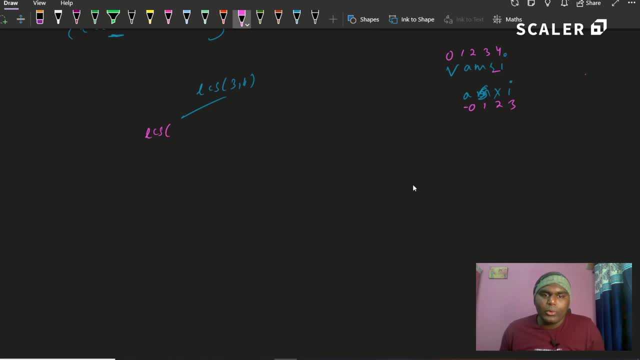 not equal. so what? what are the two choices you have? you can either move left or you can move right, okay, okay now. so two, one, one, two and one. both are not equal. again you have two choices: lcs of one comma one, lcs of two comma zero. so one comma one, not equal. okay, again you will be having 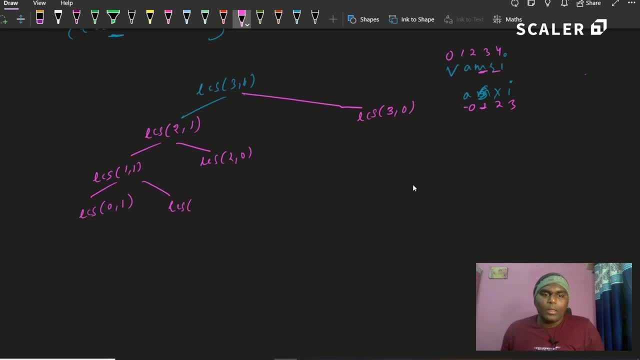 two choices: zero comma one. both are not equal, so you will say again, you will be having two choices: lcs of one comma one and lcs of zero comma one, 0. okay, so since it has seen minus 1, there is no index called minus 1, so you will return. 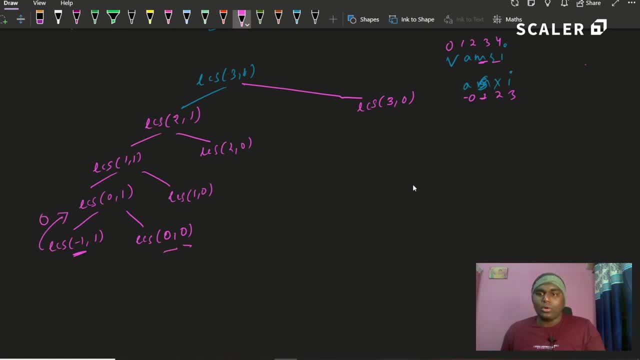 a 0 here and 0 comma 0. both are equal. no, so you will return again 0 here. okay, sorry, sorry, okay, you will make another choices: minus 1 or 0 lcs of 0 comma minus 1. so since you have seen, minus 1. 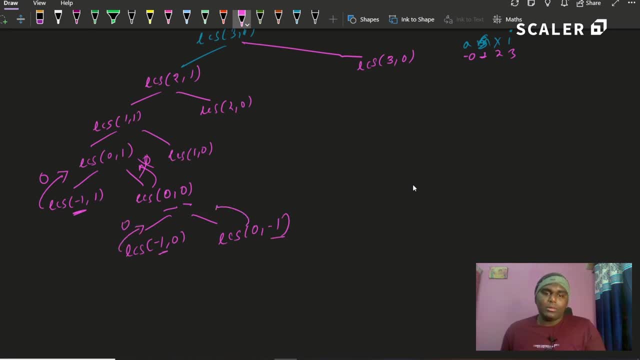 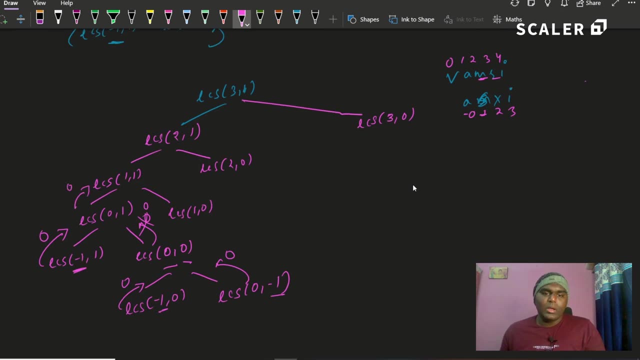 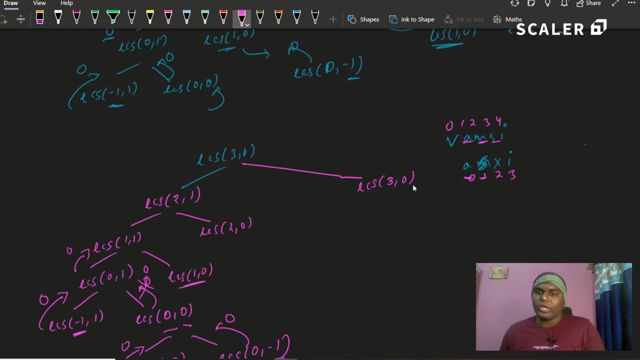 you will return 0 a 0. okay, so max among this was again 0, so it will return max a 0. now you will compute 1 comma 0, so 1 and 0, so both are equal right, a and a. so you will be having only one. 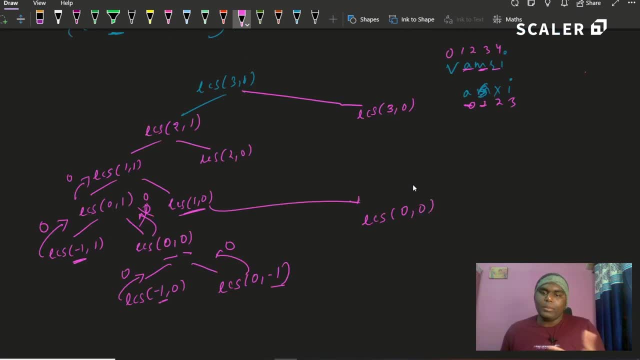 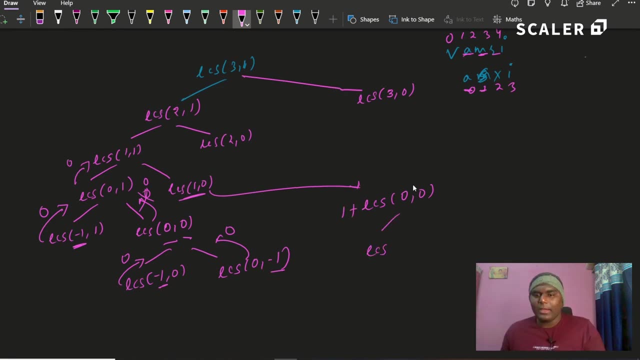 condition called both decrease of both. okay, and you will have plus 1 as well, and here 0 and 0. both are equal and no. so you will be having again two conditions: minus 1 and 0 and 0 and minus 1, okay. so since it has seen minus 1, you will return 0 and 0, okay. so 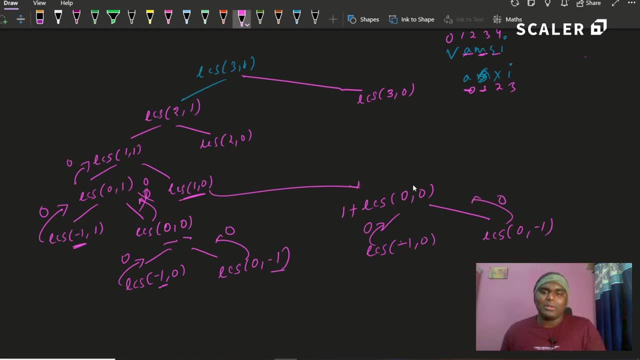 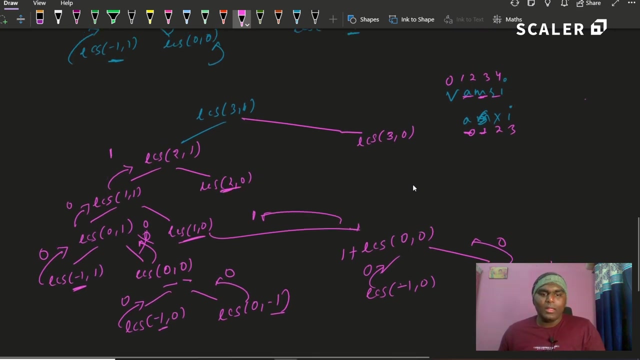 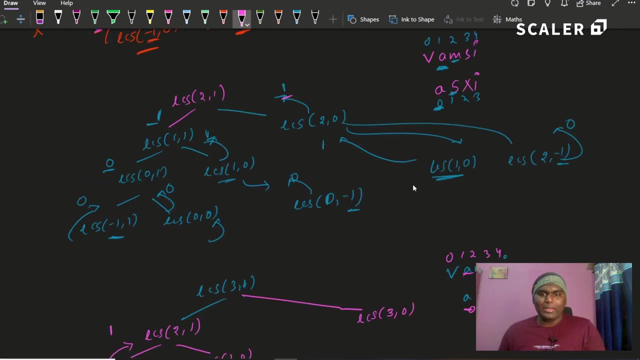 it will again written max, so it will be 1 plus 0. it is again 1, so 1 max out 0 comma 1. it will return 1 only now. 2 comma 0, lcs of 2 comma 0. so i think we have already computed that. okay, it is returning a 1 only, okay, so i'm simply gonna. 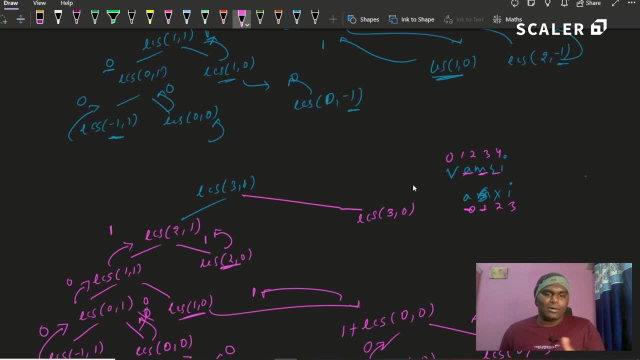 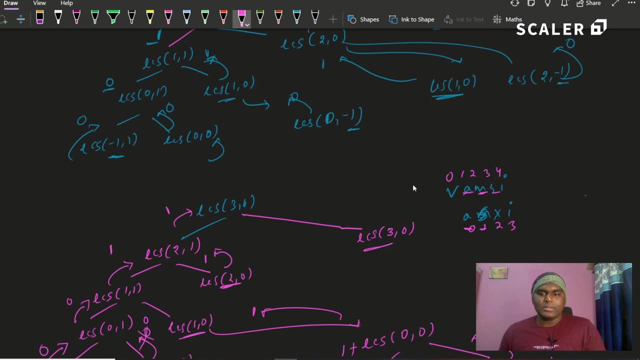 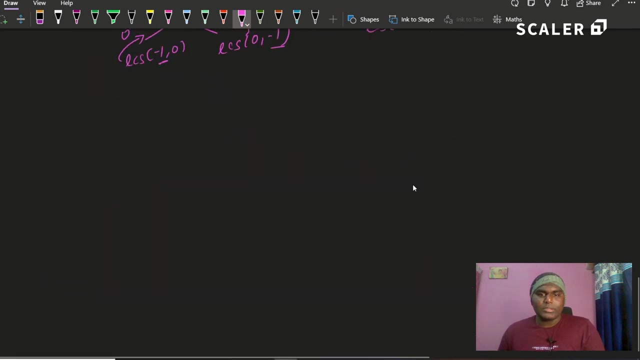 make it 1, so max of these things it will 1. and let's say lcs of 3 comma 0. so did i computed that already, did i made okay. so lcs of 3 comma 0, umc, a, s, x, i okay, so 3 and a 0, both are not equal. so again it means that i have two options. 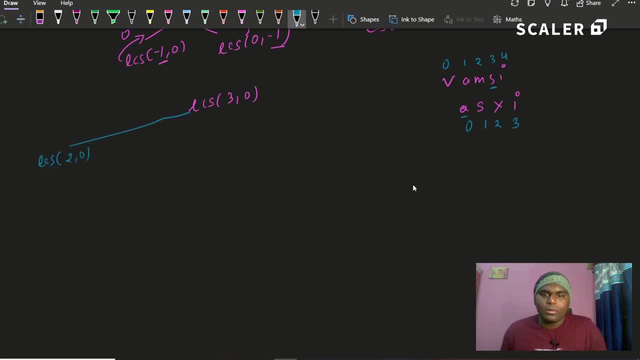 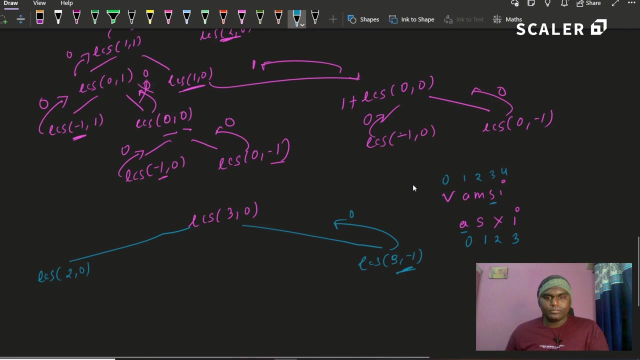 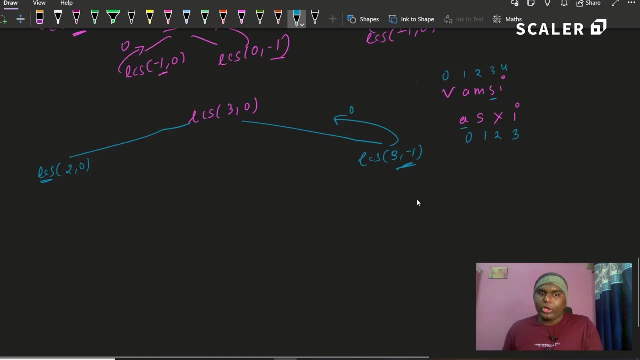 lcs of 2 comma 0. lcs of 3 comma minus 1. okay, since i have seen minus 1, i can simply say return 0. so now let's compute for this. lcs of 2 comma 0. okay, so 2 comma 0. m and a, both are not equal. yes, i have again two choices: lcs of 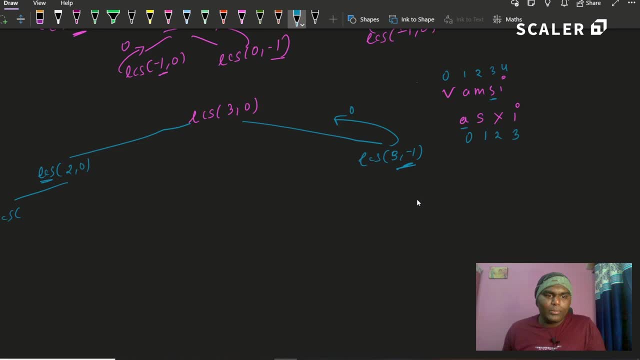 1 comma 0 and lcs of 2 comma minus 1. okay, so 1 comma 0, both are equal. yes, both are equal, so i will return a 1 plus lcs of 0 comma 0. sorry, 0 comma minus 1, so since it has seen minus 1 i. 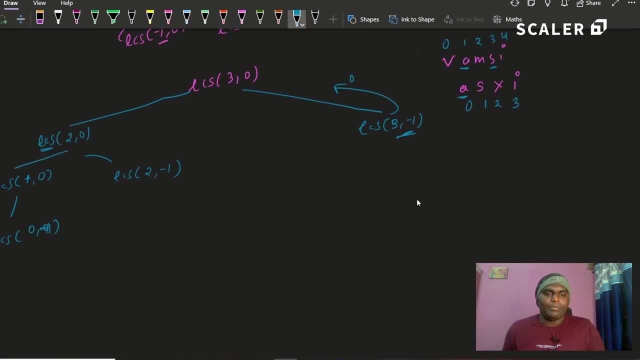 will simply return 0, so it's a 1 plus 0. it's a 1. now i will have seen minus 1 here, so i will return simply 0. so 1 plus 1 max of 1 comma 0. it's a 1, so it will return 1 now. 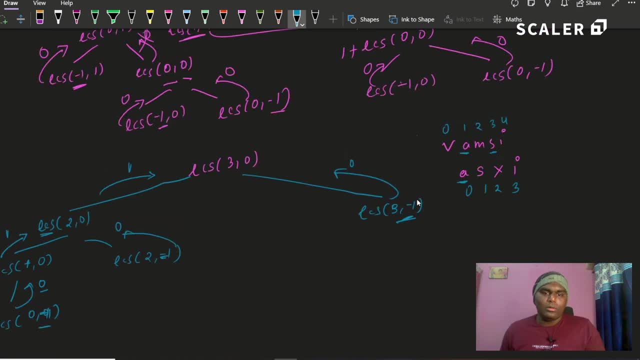 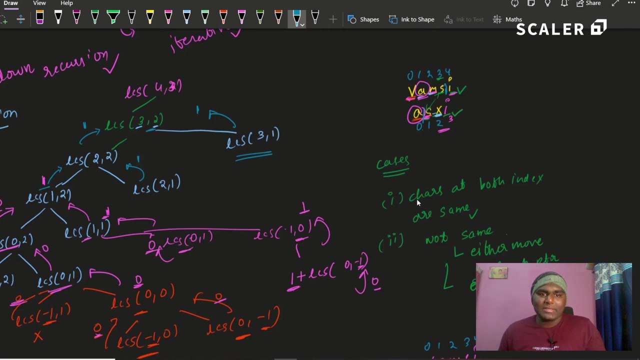 you max of one comma zero, it's a one. so it means that lcs of three comma zero returning one. okay, it is returning one, cool. now. it means that max of it will return one. so it means that here it will return one. so here, what is the max here? so it is saying that both are equal and it means that. 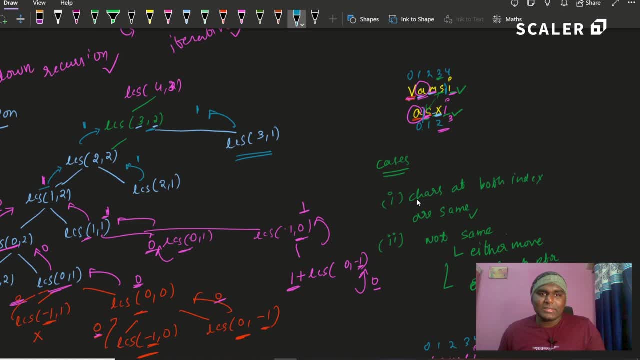 um, it will return one plus, uh, max among these. sorry, yeah, max among these, it's a one. right, it's a max among these were one. so it will return one plus already we have one. so it is a combination, right, one plus one, it's a two. 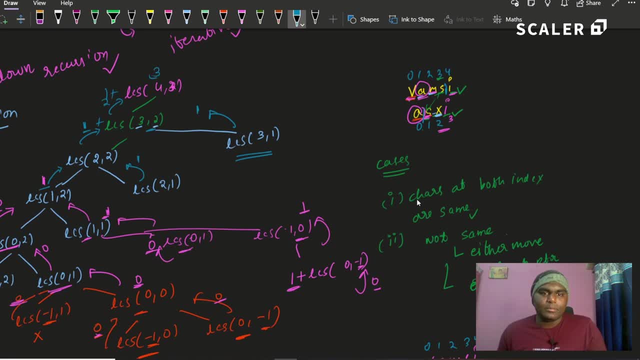 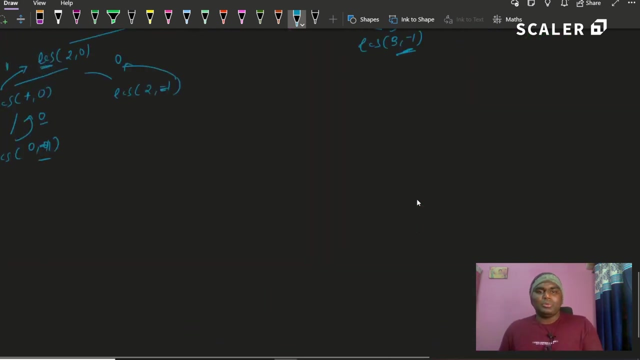 and here again you will be having one, so it's a three. so that is what the answer says to that right. a yes, i asi is a sub sequence. okay now. so we have seen all these recurrence relations. it's a little mess, yeah, little mess here, so but it's okay, okay, so we'll now try to uh remember the steps, i hope. 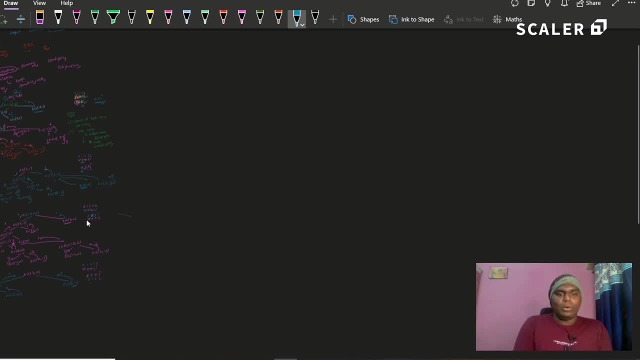 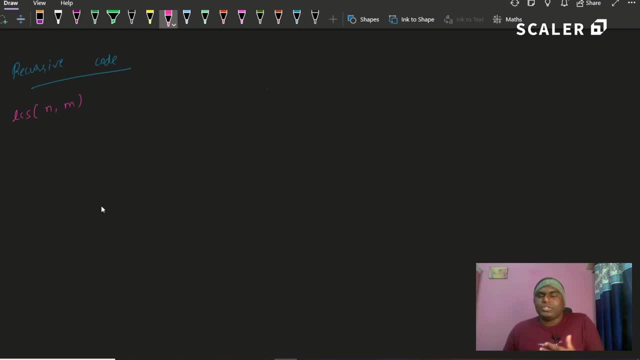 a, taking en and m, so which are both. uh, these are what will be our base condition. so whenever we have seen anything less than 0, 0, we are saying that return 0, so done. this is our base case. is there anything that we are stopping? no, now, if this is not the 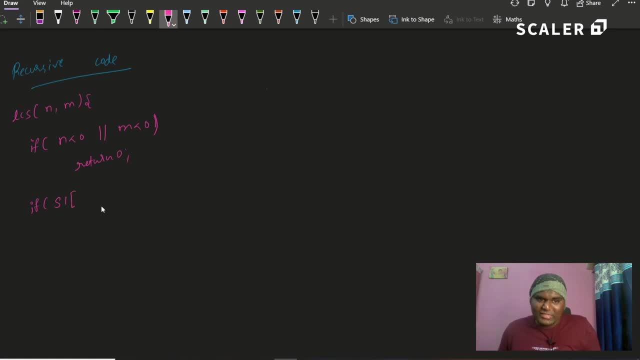 case we are checking with like s1, so string 1 n double equal to string 2 of m. basically i'm checking both the characters. so if this is the case, what i am returning i'm returning 1 plus lcs of. i'm decreasing both the indexes right: n minus 1 and m minus this is what i'm. 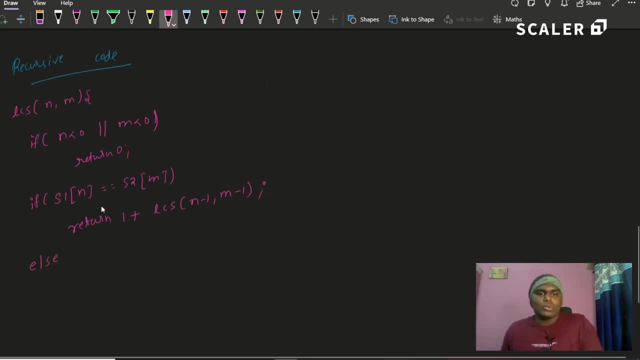 else else else, so else i have to work on this. what is move left? so i'm considering the left subtree. what is the left subtree? so i'm decreasing my first string pointer, okay, i'm not adding anything. so lcs of so n minus 1 comma m. i'm putting that, my second index pointer, at the same place. okay, and i'm 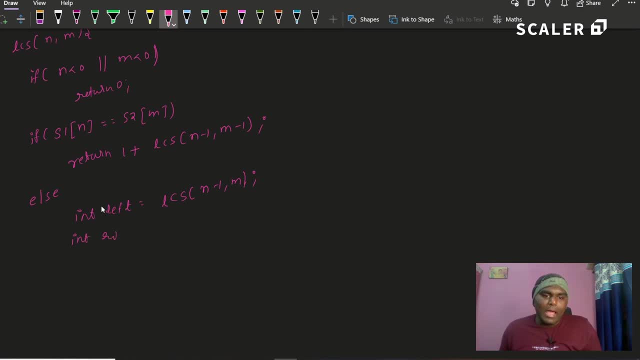 moving, and in the right i have another option called in the right, lcs of. i will be sticking at the same in this string 1, but i am decreasing my string 2, pointer. yes, now, at the end, after this computing these things, what i'm doing? i'm returning. 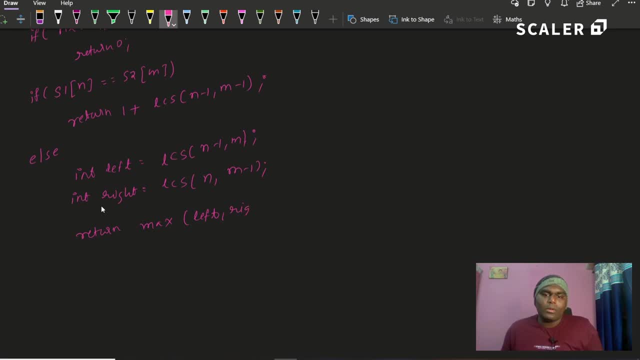 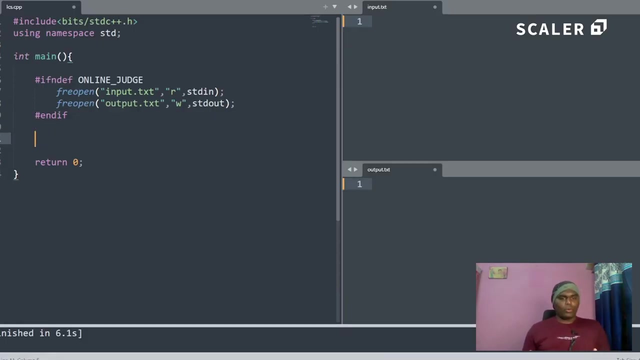 max of left and right, done so in the whole process. this is what i am doing. yes, this is our recursive code. okay, now let's discuss the code. okay, let's try to code the what we have discussed in the solution. so first you will be required to accept the input, which: 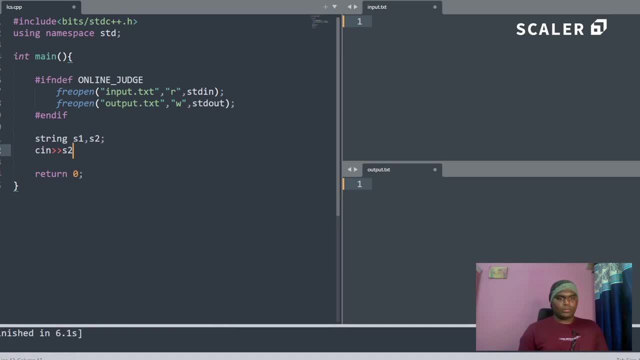 is things okay, so we'll see what we had discussed in the solution. so first you will be required to accept the input which is things okay, so we'll see that here. okay, first we have to do the same row. okay, let's see, this is the first mix. okay, first will be the second one. 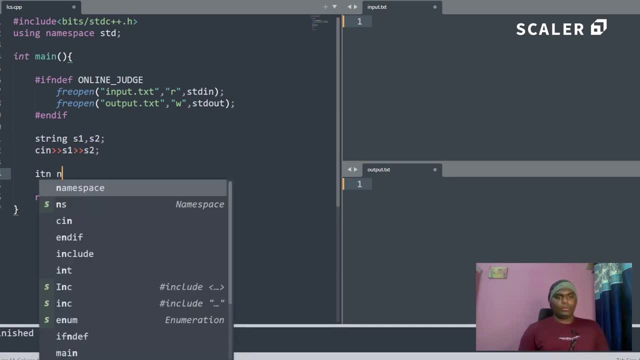 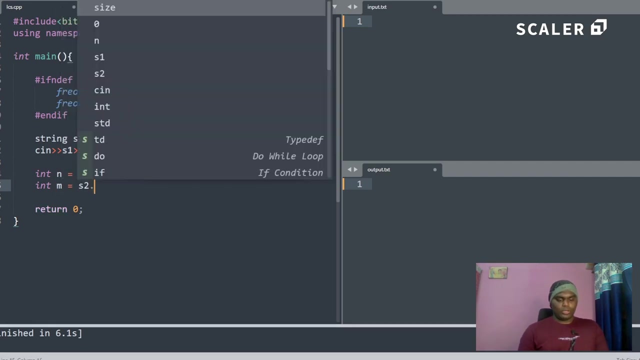 then you need to have the length of both the strings. now you need to compute your answer. i will be storing that recursive answer in my solution. answer then: lcs of n minus 1. so why n minus 1? since if you have computed size, let's say: 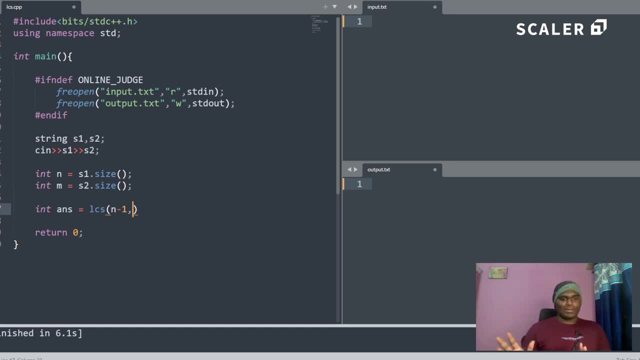 if it, if it contains a five, five characters in the string and the index would be n minus 1. so since i am starting, uh, write a start for like end from end of the string. it will be n minus 1, then m minus 1, s1 and s2, so at the end you will print that answer. 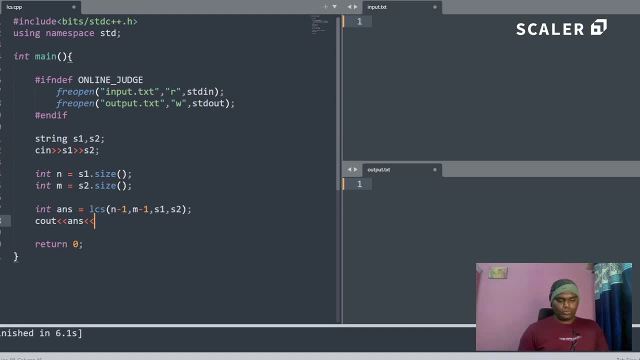 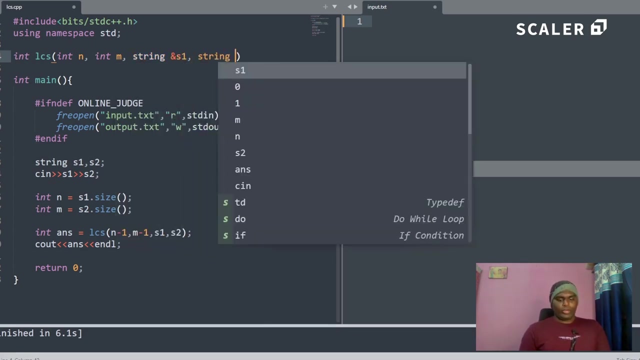 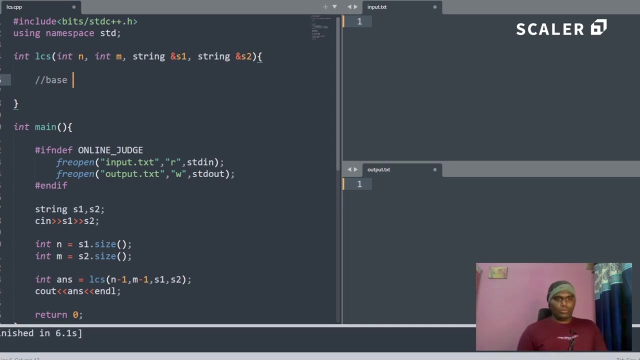 so you, let's try to go on. create the. it will return int. okay, it will return the longest common subsequence and you will be taking n in s1. first you need to write the base cases. what are the base cases? so if either of my indexes, if either of my indexes are less than zero, 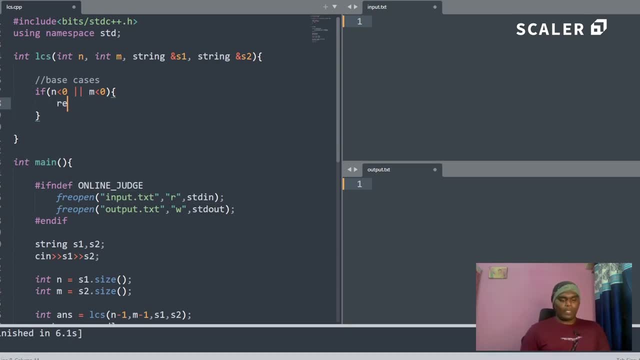 either of my indexes are less than zero, i need to say, and at zero. that will be my base case. if, if this has been the not the case, i have to consider the case one. so, if you have remembered, we will be having two cases. first case is when my string like character. 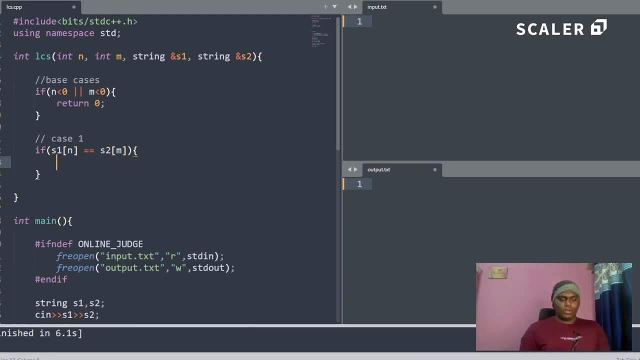 both the characters are equal. if both the characters are equal, what i am doing, so i will just reading: one plus- i'm moving both my pointers down at the same time- and minus one in minus one: s1 and h2. this is not the case. what is the case two? so just, 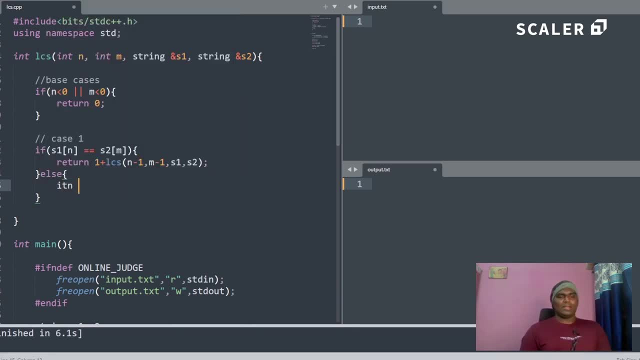 you can consider: uh, you will be taking a left, so left sub tree, okay, what will be the left sub? so i will be moving my first pointer down, which means that n minus one, and i'm keeping my m same at the same position where i'm currently now. so 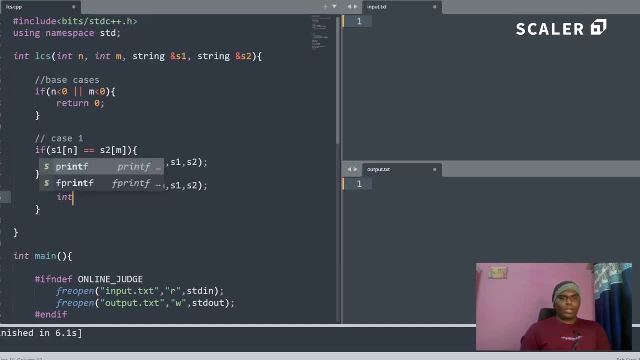 one and s2. i'm moving at my right, a sub tree lcs of n comma n minus one s, one comma s2. so at the end, what i'm doing, i'm just returning max of these left comma, right? so this is what i'm doing, right? 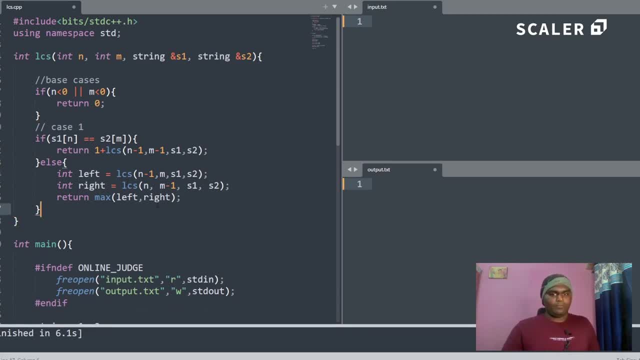 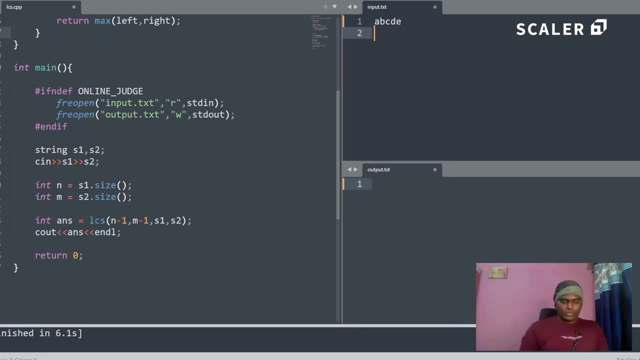 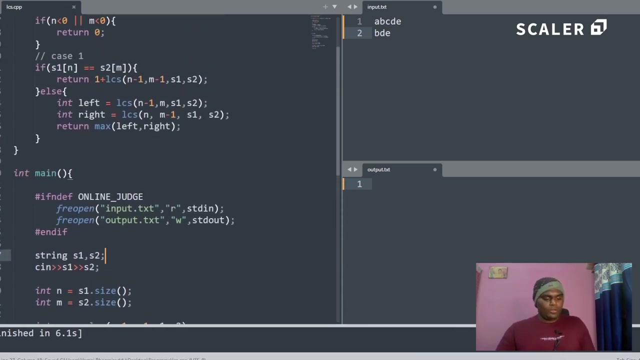 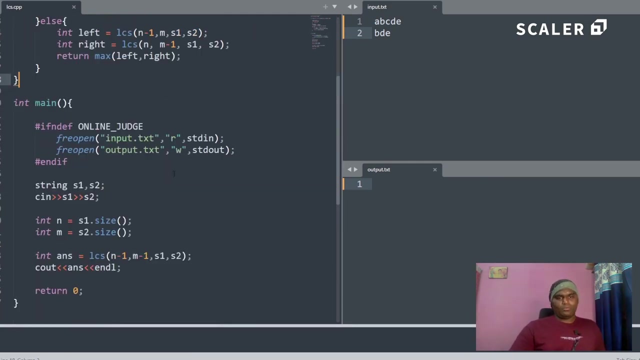 so let's simply try to run this code, okay? so, oh yeah, let's do some inputs: a, b, c, d, e was a, b, d e. answer would be three here, right? so yeah, the answer is building hope we will get the answer. so i'm unable to see any errors, though. 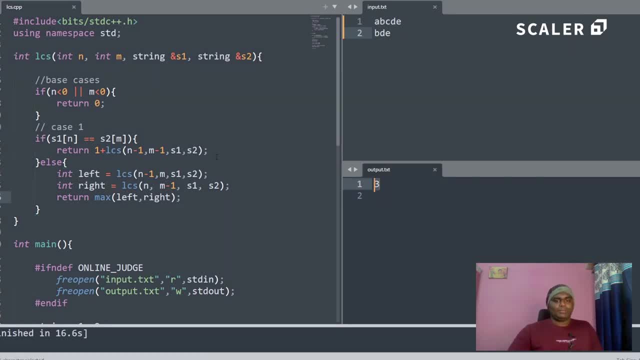 yeah, this answer is three. we got it. we got it now. um, um, let's try to figure out the complexity of this particular approach. what will be the time? complexity first. so here. so we'll be having a three loops, but it's an if and else, so i'm pretty. 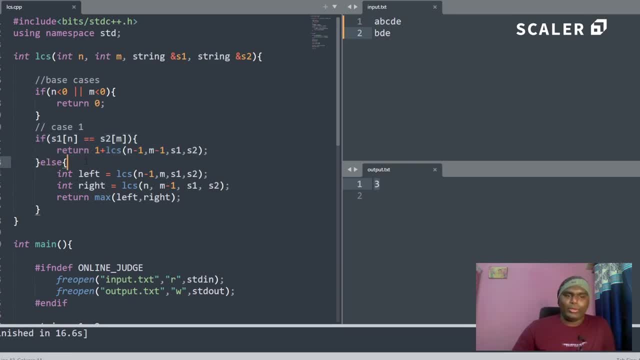 much sure that either either of the block will be get executed. so, and uh, you have to consider the max scenario. so let's assume you have, uh, been calling always two calls. okay, so left and right. then you will be having two choices. okay, for each combination you will be having 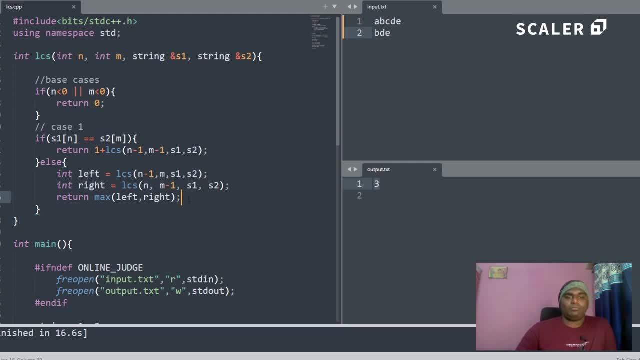 two choices. okay, how many combinations you have? okay, so let's say uh. when i say combination, so you will be having, let's say n as five and m as uh, three. okay, so, how many index combinations you have? uh, you, can i say a zero comma one? can i say zero comma two? can i say zero comma? 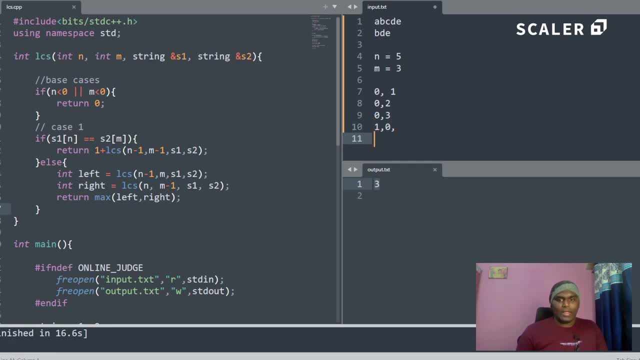 three and one comma zero. then, uh, one comma one, then one comma two. so for each and every number you will be having three. so for such that you will be having n into m, m into n combinations. it means that the complexity of this particular approach would be. 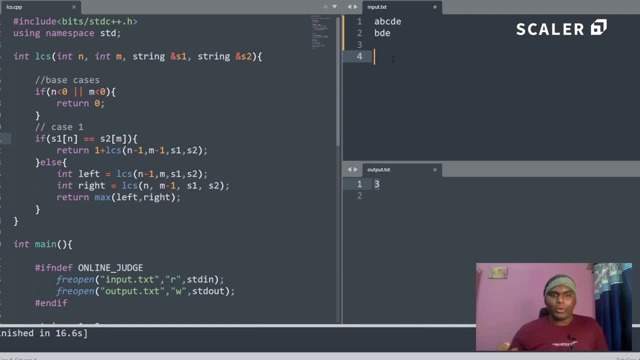 two power n into m, two power m into m. so you will be for each and every combination. you have to uh choices: either you have to go, you can uh go left, you have to go right. okay, we'll be moving both. and you are saying this is not right and this is right. so 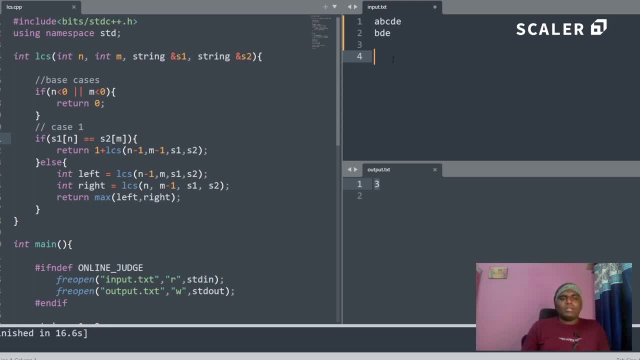 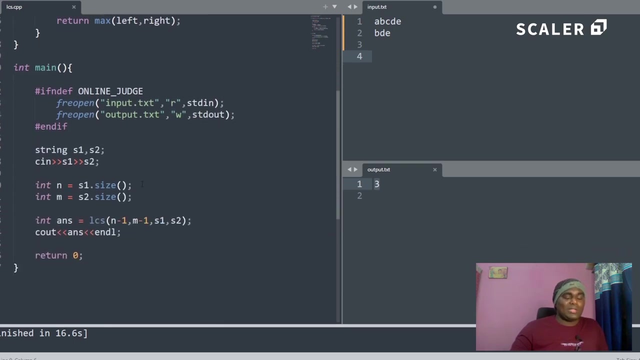 you are computing like that. so can i say that complete overall complexity of this approach as a big of uh two into sorry, two power, i mean, yes, i can, and what will be the space complexity? so we are not using an extra place, but we are using an auxiliary space called stack space. 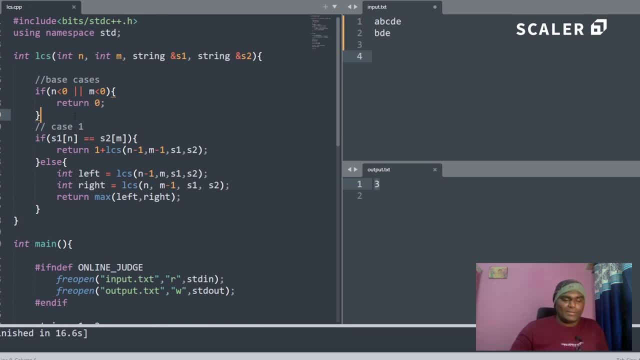 as you all know, that recursion takes a stack space. so what will this pack stack space here so that stack space is uh, again big of um two power? i mean doing that many combination that we are trying right. so is that a like uh, since it's an. 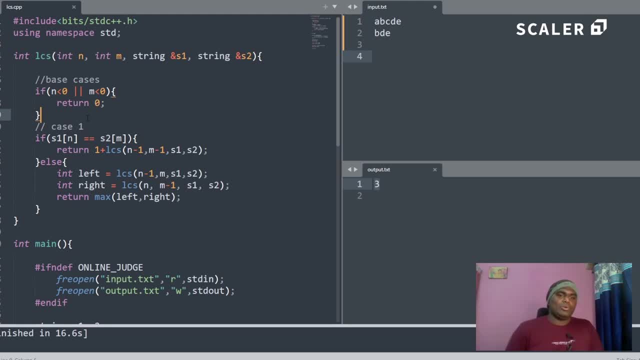 exponent. this is not an accepted solution. so the interview will ask you to optimize that further. so whenever you have written a recursive solution and you got to, you have to optimize that solution. then you have to remember one thing: you have to do with that with a dp first. 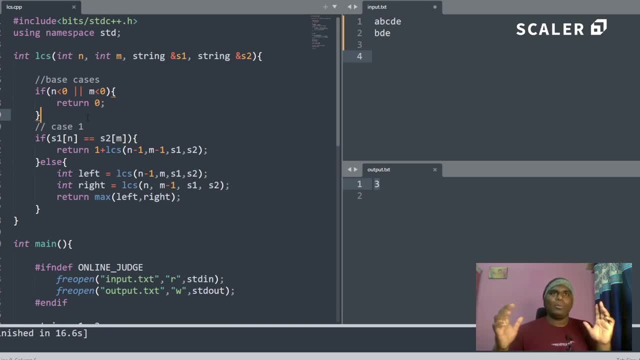 okay, dp. so if you don't have a much time in an interview and if you felt there are some other solutions, as like bfs or any greedy approaches, that is, are lower than a dynamic programming or recursive, then you can go ahead and explain it, because, basically, uh, explaining dp, uh like solutions to an interview in an 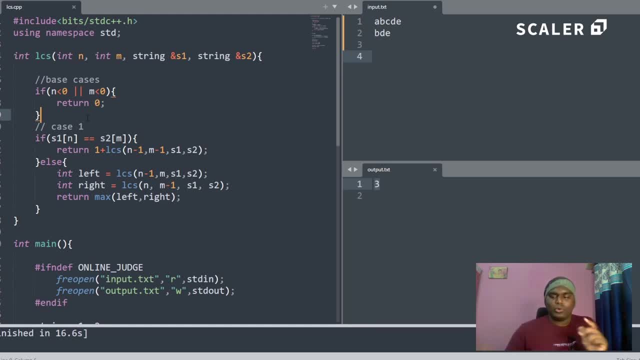 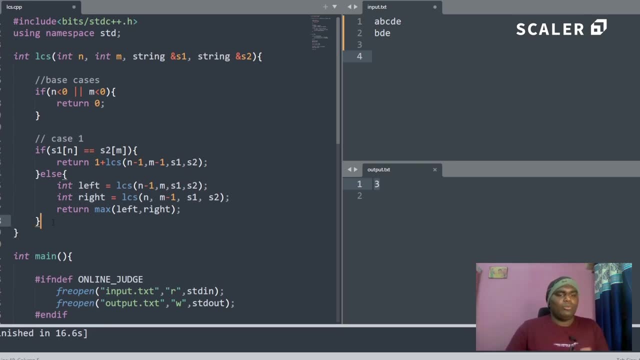 interview. it takes a lot of time, it will kill a lot of your time, so i recommend you to directly jump into another solution if you have any other solutions in mind. now here we don't have any other choice, so we have to do it with a dp, so we have a recursive code. so now i will tell you. 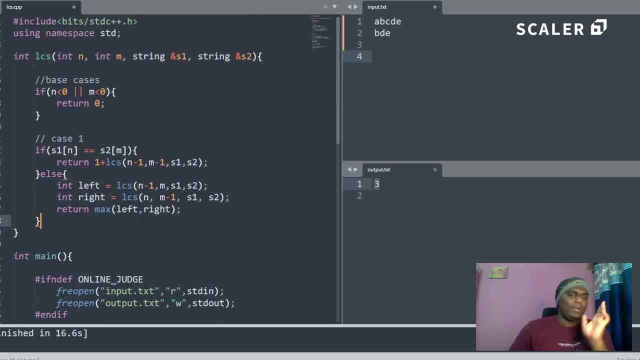 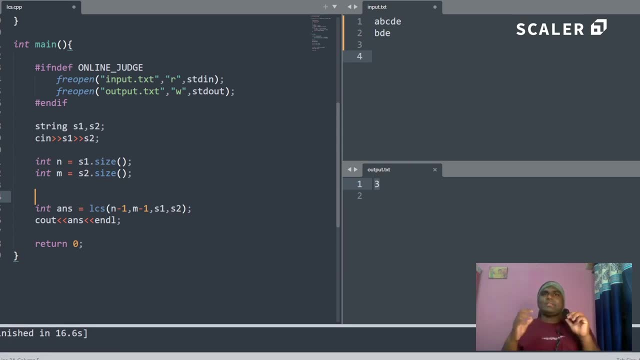 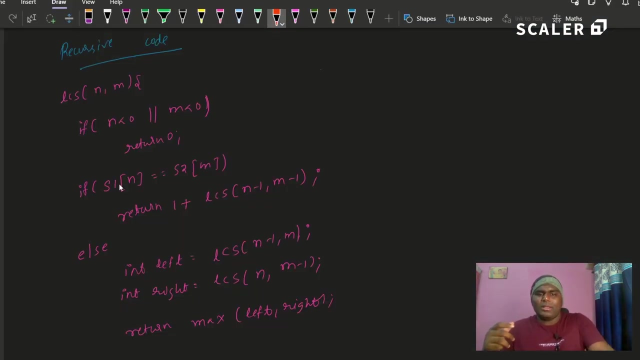 how to uh, convert this into dp, simply. okay, that approach is called a memoation technique. okay, i will tell you that. so what is a memoation technique? so basically, memoation means like, let's say so, um, let's see first, first so, whether we can do this problem with dp or not. so i will tell you that. when can we go with dp? 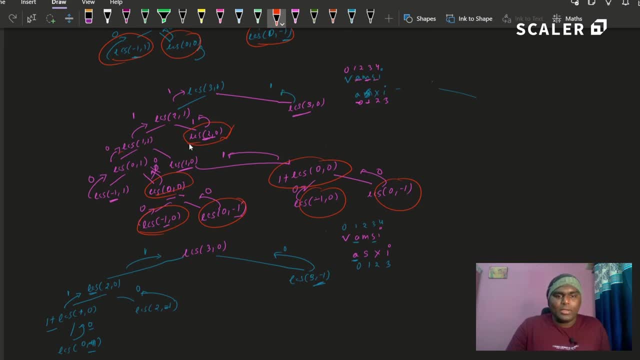 so, as you can see, here i have highlighted few things. so lcs of lcs of two comma zero and zero comma zero. so again what you can see. so i am computing lcs of zero comma zero two times here. so are you pretty much sure that i am computing only. 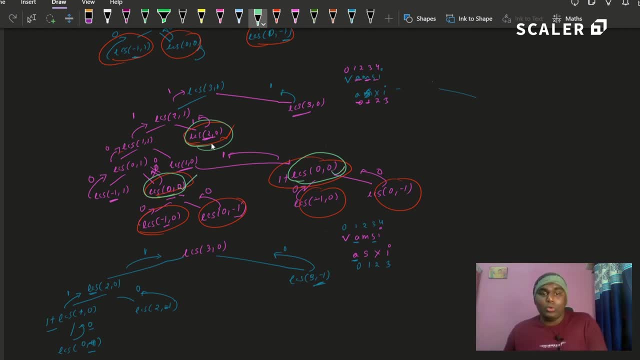 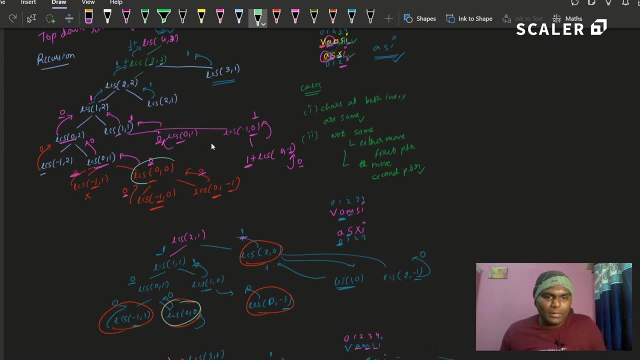 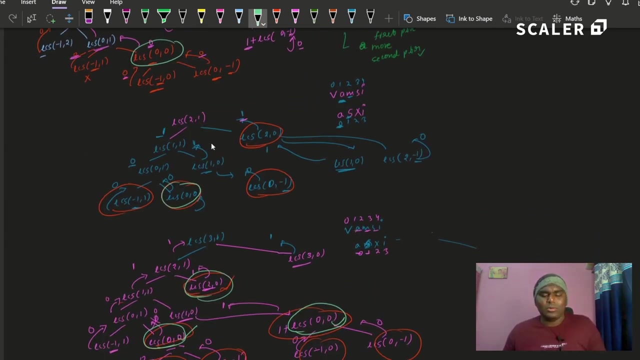 two times. no, let's say so. i am computing zero comma zero here, okay, and if i go up again, i am considering computing zero comma zero, right? do i need to compute these many times? do i need to compute these many times? no, so the answer of zero comma zero was zero at any time. 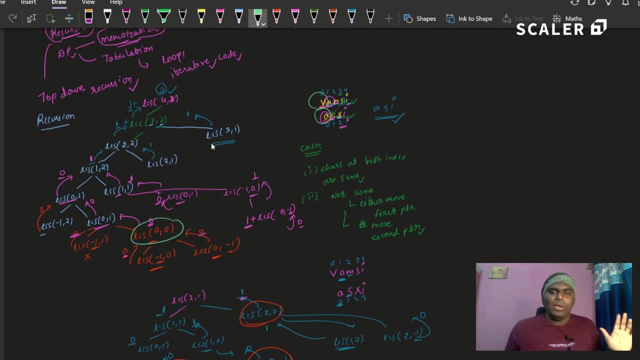 because v and m were not matching. so whenever i have computed zero comma zero, the answer would be zero only. okay, so for that do i need to compute that many times? no, so now think: okay, imagine if something happens like this. so uh, whenever i have computed, i have solved some uh sub problem. okay, i. 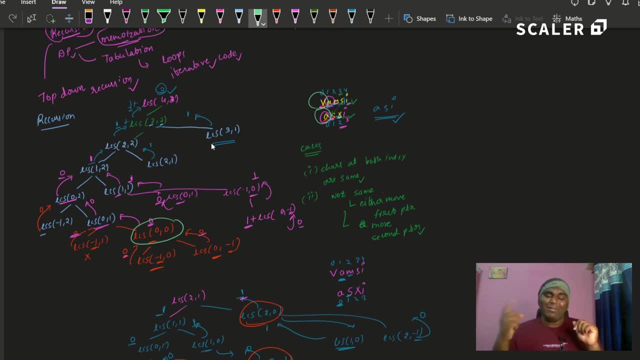 will keep that in my memory, okay, so whenever again i'm- uh, i have asked me to. okay, i have asked my mission to compute that particular problem again, so my mission knows the answer. okay, what he, what my machine can do again? it can simply return the already previously completed answer. 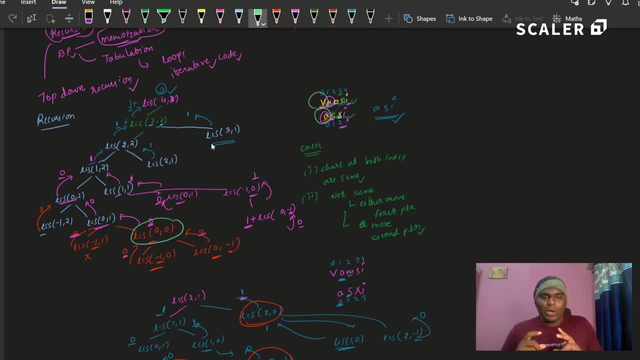 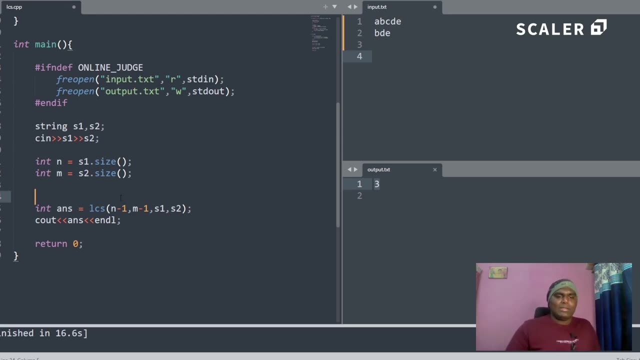 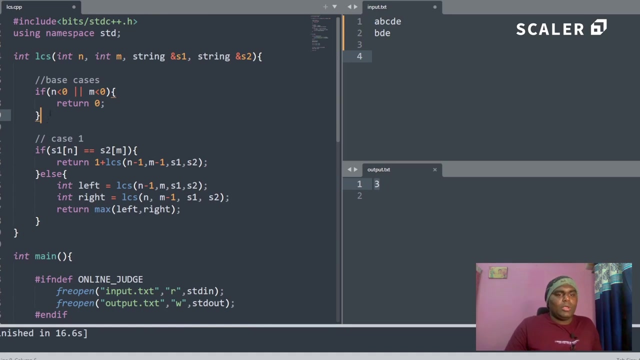 so this is called a dp and this is called an dp. so how can we achieve dp using these recursive calls? so i will be first telling the memoization: uh, let's take a vector of vector. so, before moving into that, so how much space that we i need to assign? so that will be my first question. so how? 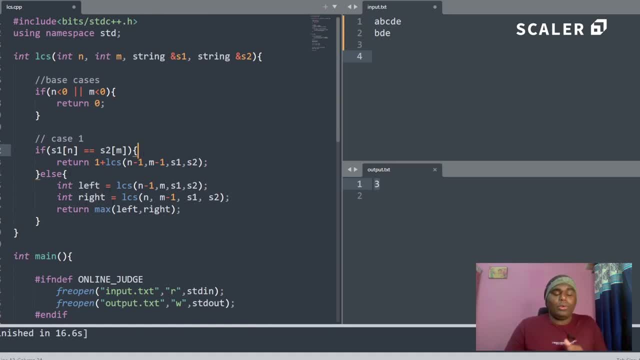 much space that we need. so here you for that. you need to observe what are all the changing factors, like changing indexes. okay, what are all the values changing in your recursive code? so here my change values are m1 name, so it means that i need to memorize these both. i need to keep that in my 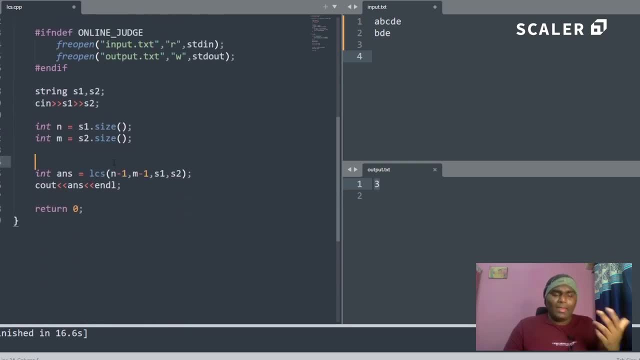 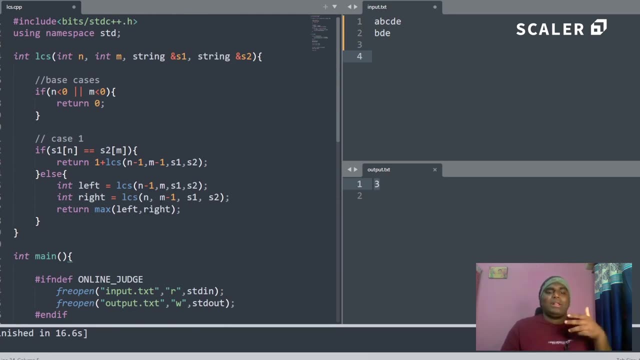 memory. okay. so if so, here, uh or two values are changing, i need to consider two dimensional array or vector. okay. so if a three indexes, like three values, are changing, then i need to consider three dimensional vector or three dimensional array. okay, if one index is changing, now one value. 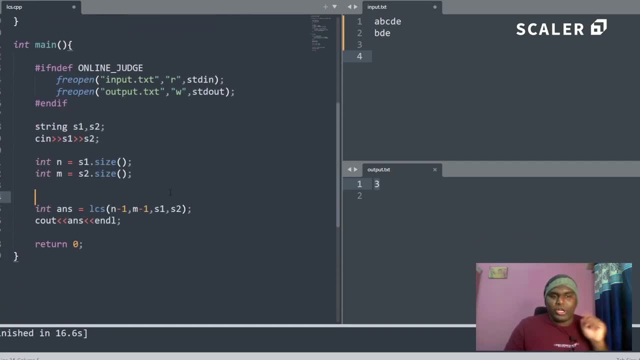 is changing, then i can consider a one uh dimensional array, all right, so i need to keep that in my memory: m, so here 2. so I will consider two dimensions, so vector of vector dp of n into m, so I will be initializing that with the minus 1. okay, so why minus 1? let's say I am putting that: 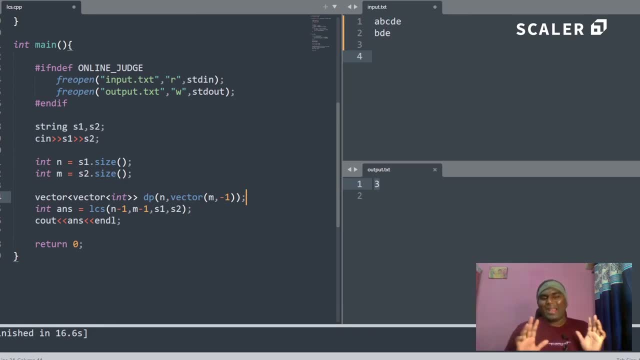 minus 1 as an my empty space. okay, empty space, I haven't solved any problem. so whenever I am my particular space, my particular problem is not minus 1. it means that I can say that I have the solution for you, okay, so I will simply return that, that's it. so I need to pass here dp as well. 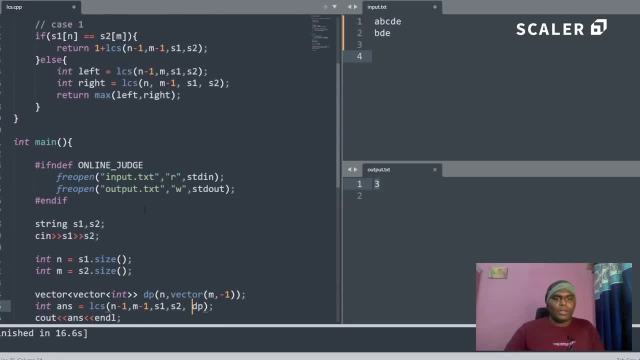 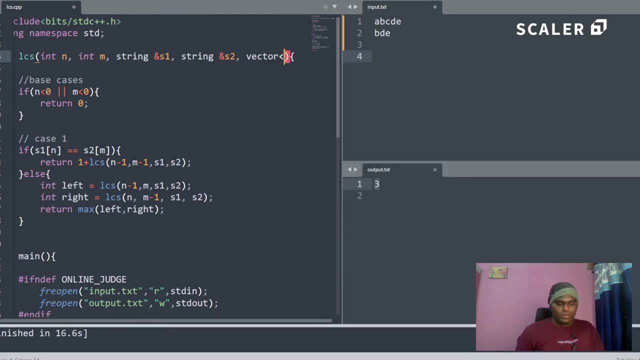 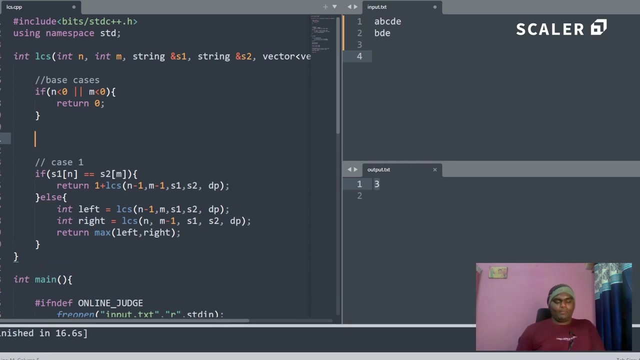 as my parameter for argument, I will go top and I will implement it in my uh. I now uh. so wherever fun I am making a function calls, then I have to make here and here now what I do. so here. let's say, if dp of n m not equal to minus 1, 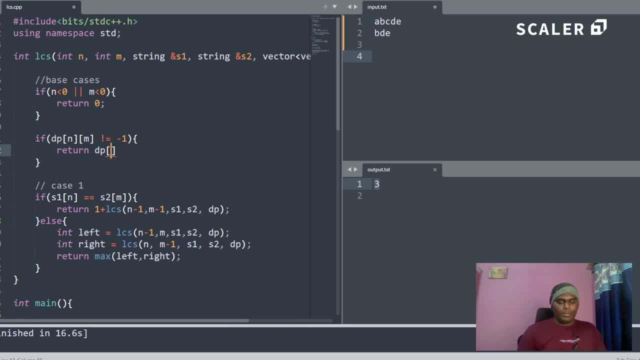 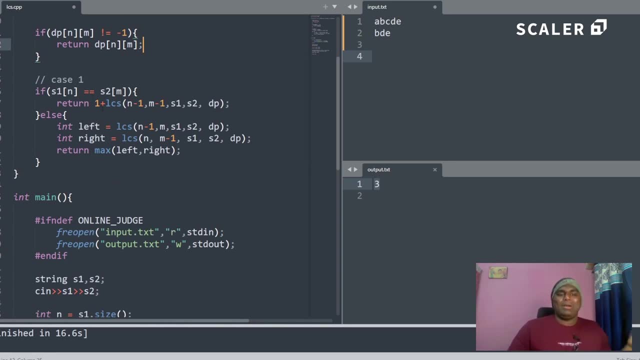 not equal to minus 1. so I will say dp of n m not equal to minus 1. so I will say dp of n? m not equal minus 1. then return dp of n. oh, I'm returning, so where I'm storing the answer. so here let's say so, instead of returning your. 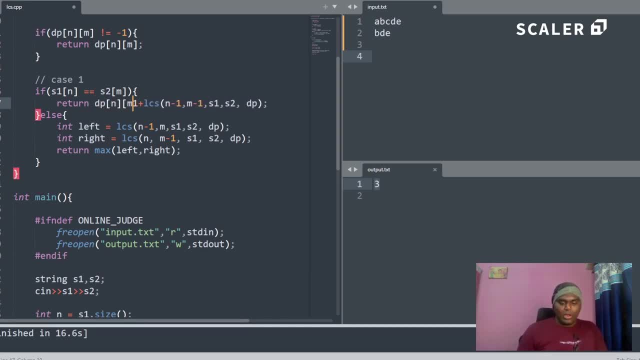 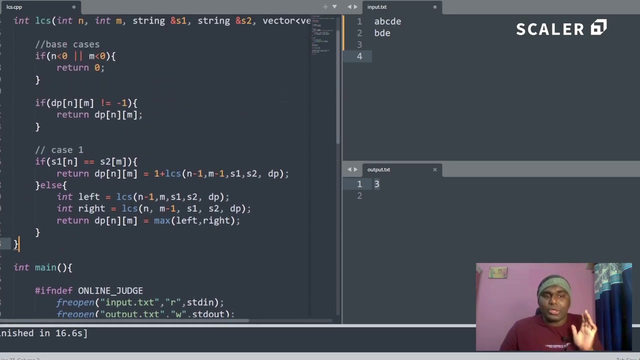 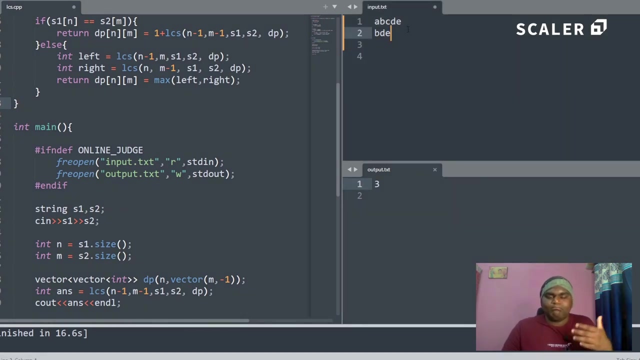 answer directly what you will do. you will store that in your answer, okay, so that someplace okay at your indexes. then you will make a call to the next one. okay, so this is how I'm memory solution looks like. okay, so let me simply uh, change my inputs then. um, let's try to run that. 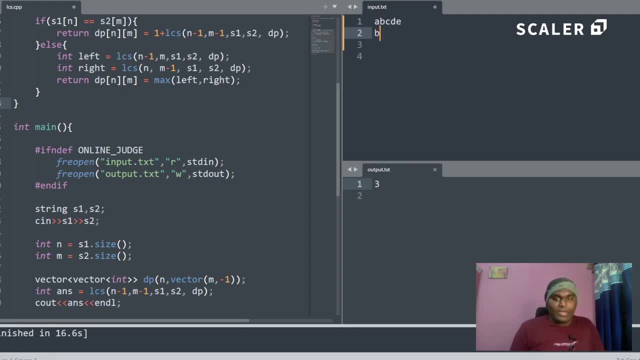 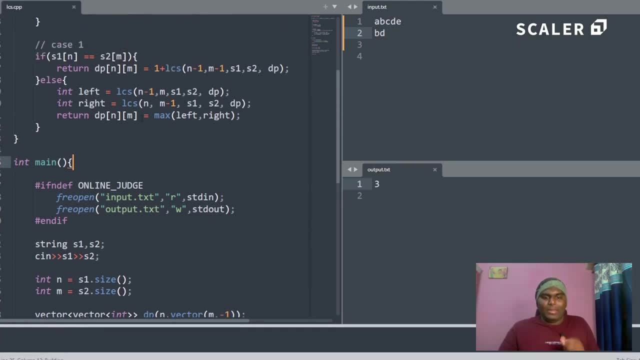 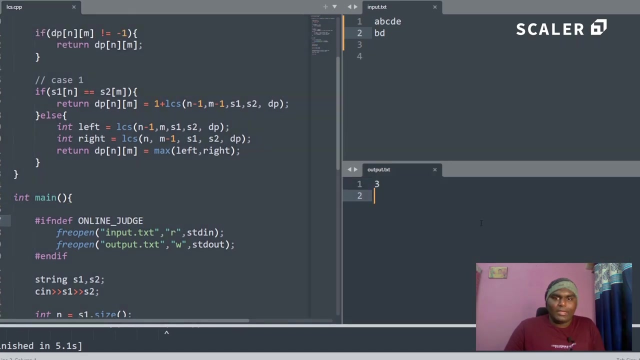 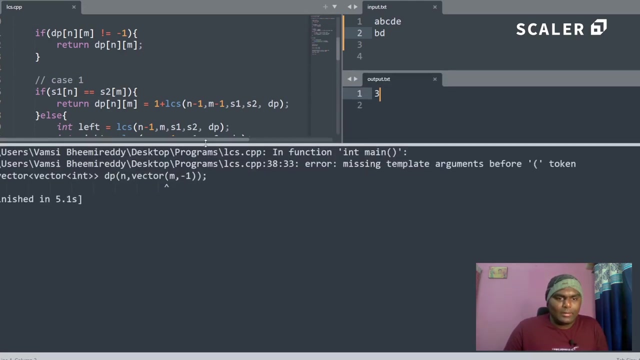 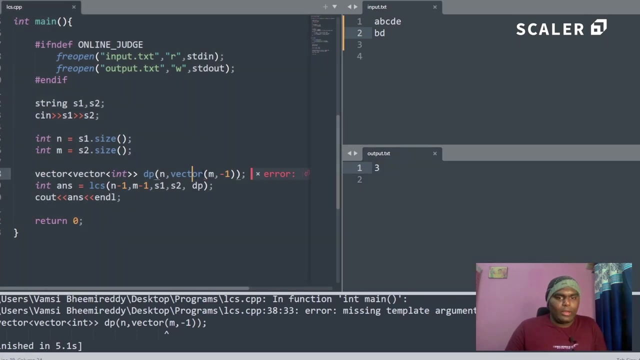 code again. so here let's say: bd, okay, bd. so now my I'm expecting to as my output, okay, let's save this and build this solution east, and we haven't got the answer. as a two it is giving okay, it is saying that there is some error. 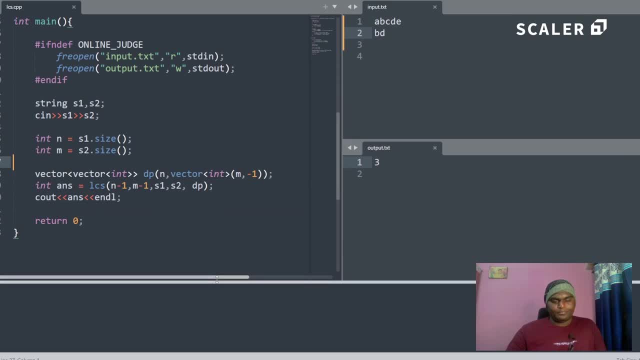 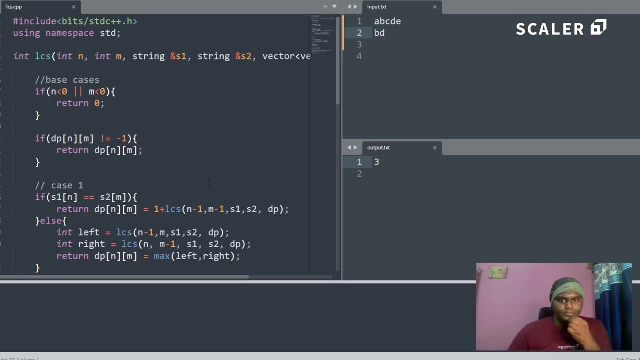 so let's try to run this one. okay, so let's try to run this one. so let's try to run this one, and what output is two. so this is how we can convert our recursion solutions to the dynamic programming solutions. so now let's try to analyze. 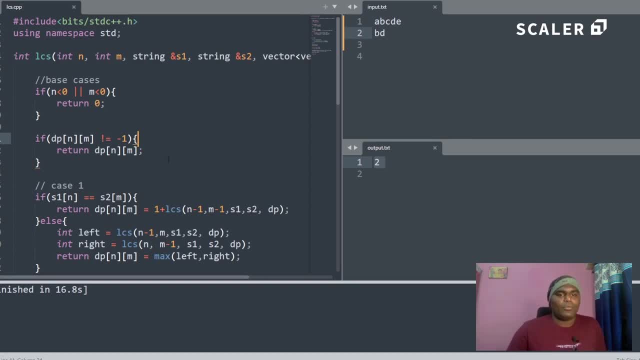 the time complexity and space complexity of this approach. okay, so what we did is we have a what we did. so basically, earlier we are making a particular call so many times, so we have reduced with that and we have memorized the answers to compute only once. now tell: 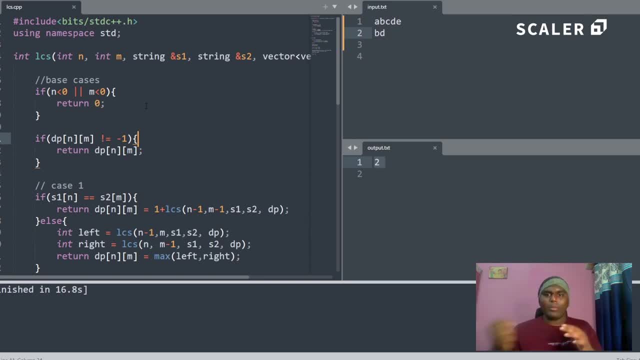 me how many combinations that we have. we have n into m combinations and how many function calls we can make. now we can make. can I say we are making only m into n combination, like function calls, how, how, how? let's say I have made one a function call once, like let's say: 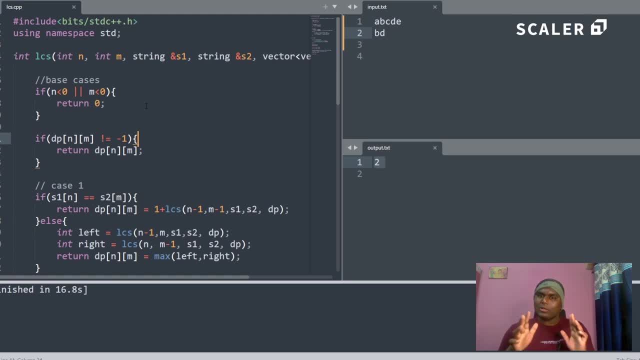 0 comma 1 and I have computed that and I have stored that answer in my memory. whenever I am going to compute that 0 comma 1 again, it is going to tell me I have already computed and take this answer, okay. so in that case, 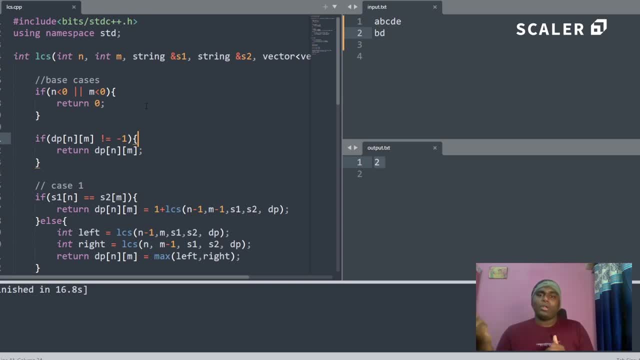 I am reducing my function calls, so I am computing only m into n, exactly all the new combinations, all the unique combinations. okay, so so that time complexity of this particular approach would be big of n into m. now coming to space complexity, so we are creating two dimensional vector. 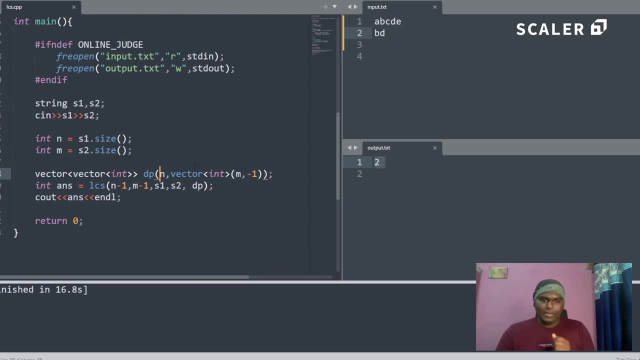 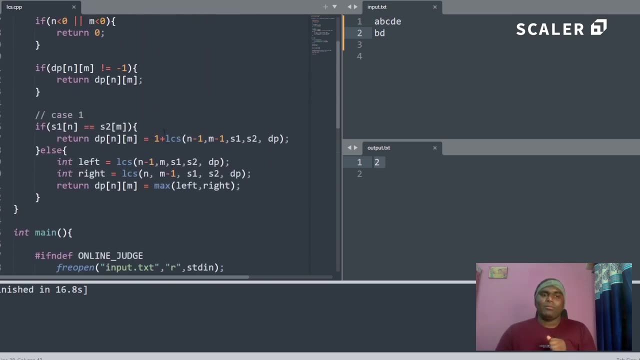 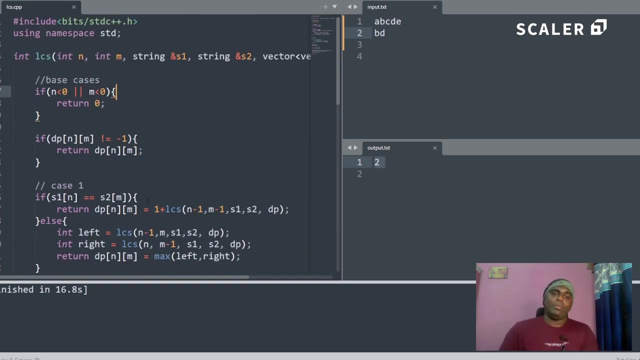 this size of m. sorry, n m, okay, n into m, so n rows and m columns, so n into m. so the space complexity of this approach will be big of n into m plus, since we are making again recursive calls, it would be again. so how many recursive calls we are? 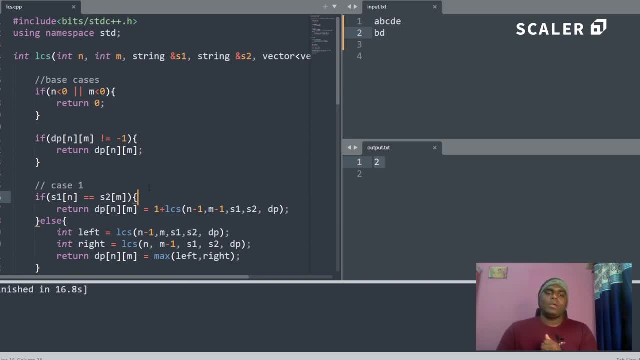 making. we are making big of n into m, okay, so, yeah, so it's so, bro, we have converted our solution to the dynamic solutions. is that enough? no, I guess. so, as you all know that recursive solutions are not that much efficient as it seems. okay, because it is using auxiliary space. 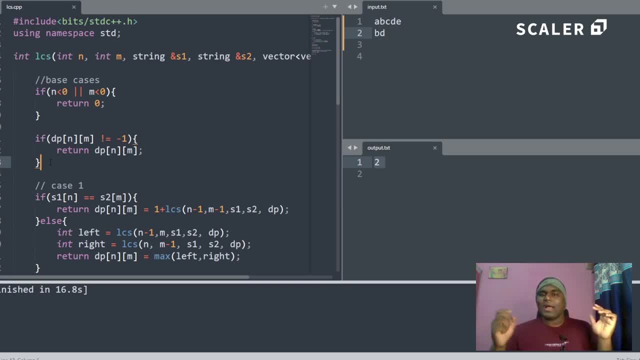 called like stack space. okay, so can we avoid that extra recursive like stack space? yes, we can. how converting like writing: iterative dp called a tabulation. so just keep this code in mind. okay, I am not using anything apart from this. I will be just writing these steps again. okay. 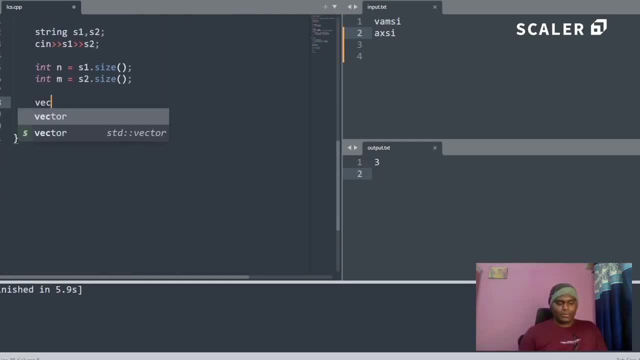 but simple amount. okay, let's try to write the tabulation method. so again, we will be required to create two dimensional array of n plus one size, this time zero. okay, I am using all with zeros. then I require: if my s1 of i equal to s2 of 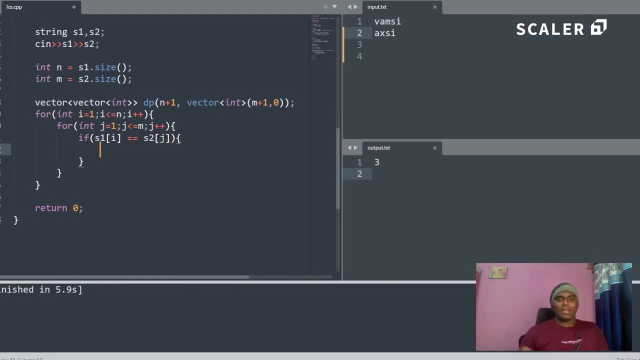 a j means that if my both the values are equal, what I need to? I need to store dp of j equal to one plus dp of i minus one and j minus one. okay, this is not that case. what I need to do, I need to store j minus one. 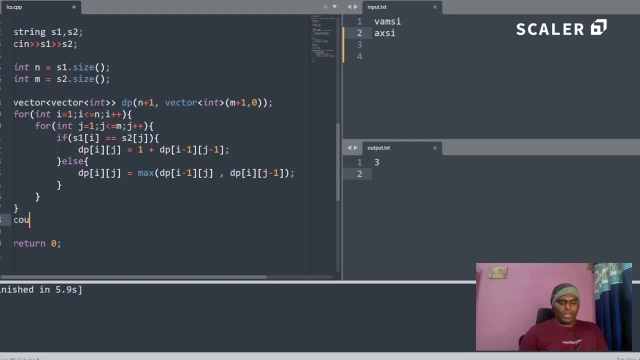 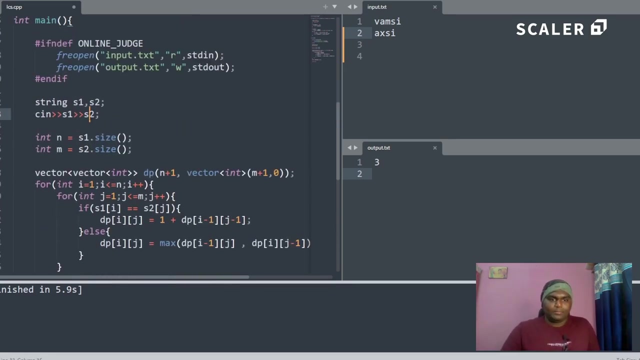 and I will return. I will printing. I will be printing c out of d of n and j minus one. okay, now let's see. the expected answer would be three, this particular output, and let's say yes, so we got three. only this is correct. okay, so now let's try to. 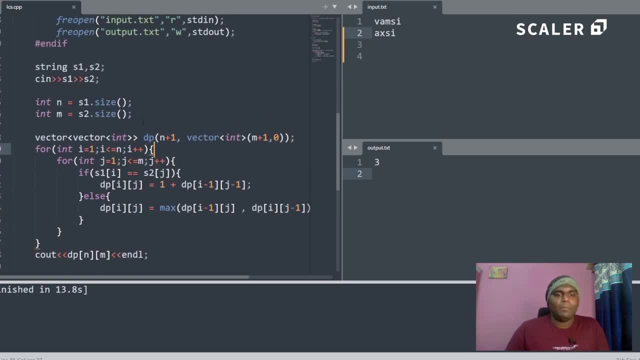 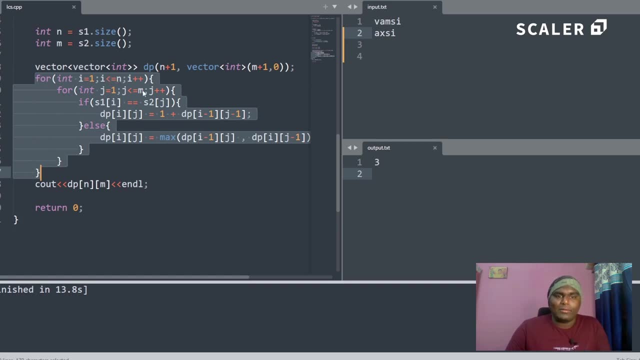 analyze this time and space complexity of this particular tabulation method. so here it's very clear. okay, so n into m. so we are using two for loops, one with size of n and one in size with m. so it's simply m into n. apart from that, we are not doing any. 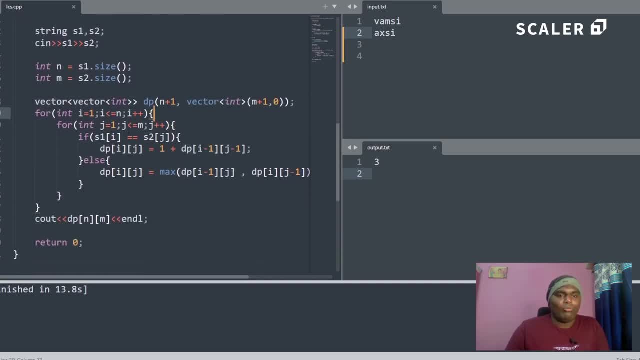 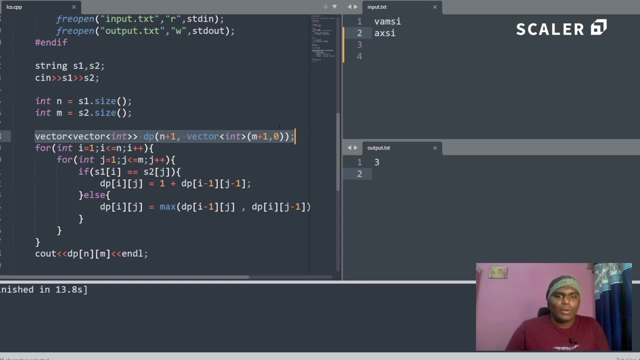 extra computations here. so the time complexity is bq of n into m. coming to space complexity, we will be creating two dimensional vector with the size of n into m. okay, at max. okay. so the space complexity would be bq of n into m. so are we creating any extra space? no, 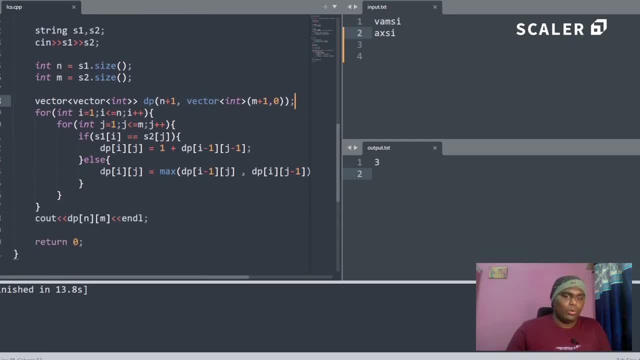 or are we have any stack space here? no, okay, so this is the difference between memorization dp and tabulation dp. in some platforms, if you submit memorization dp solution, it won't accept because you, as you all, know that it's an stack space, it consumes stack space. so if 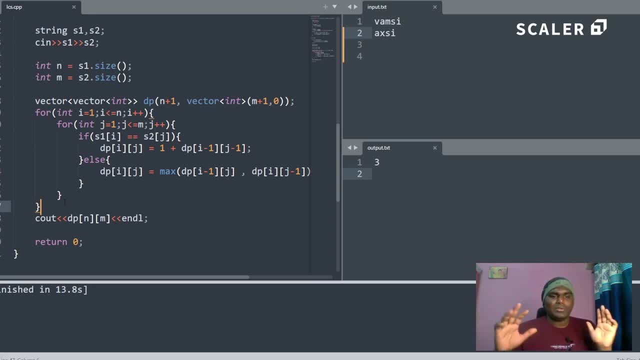 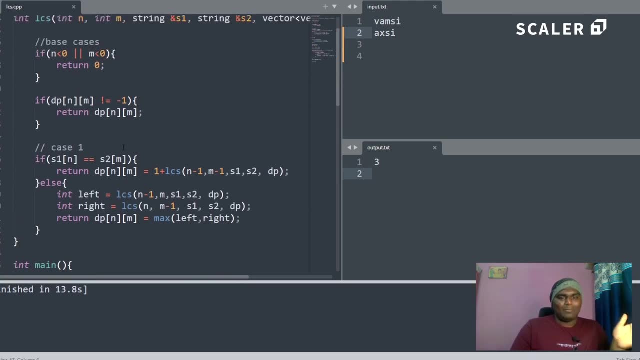 you could submit this tabulation method. it will accept. so you can see, right. so there is nothing much differences between both the solutions. okay, both are. everything is same. okay, both are same. okay, no need to worry about that. you can easily convert your memorization solution to the. 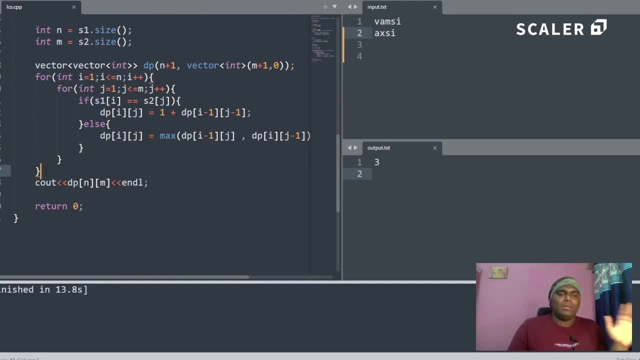 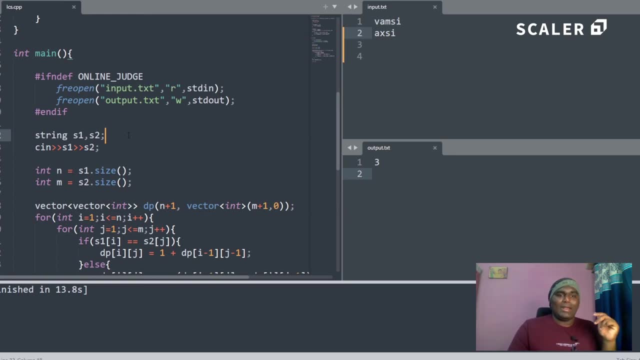 tabulation method, and if you could submit this tabulation method, it will get accepted. okay, done so happy coding. see you in the next tutorial. bye.